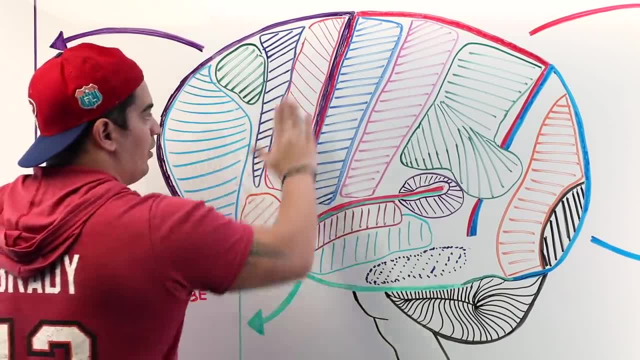 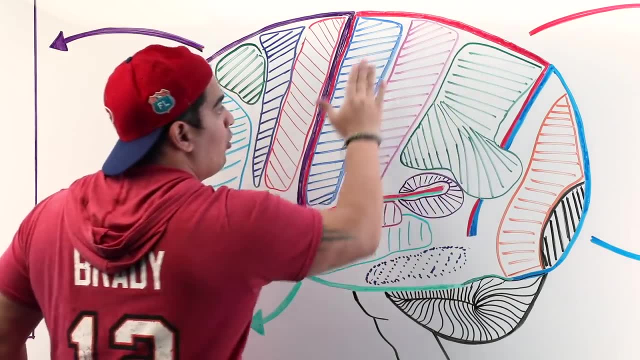 So if you imagine right here, this lobe right here is called your frontal lobe, This lobe right here is called your temporal lobe, This lobe right here is called your parietal lobe and this lobe back here is called your occipital lobe. Now we got to take it a step. 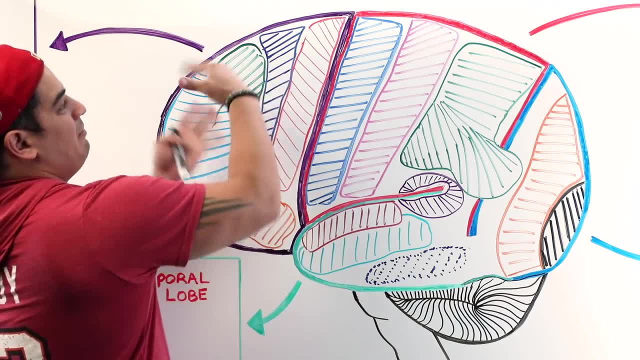 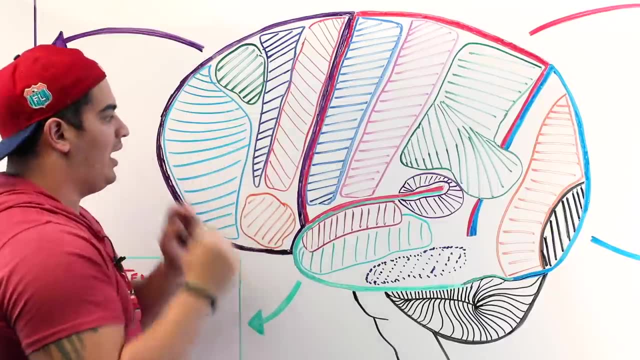 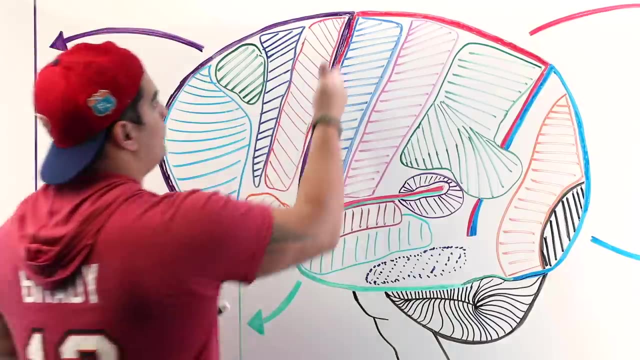 further right, because all we have is just where, maybe in some space where the frontal lobe is, We have these beautiful demarcations, or sulci, if you will, that separate these lobes from one another. What are these demarcations or sulci? This first one is beautifully placed right here. 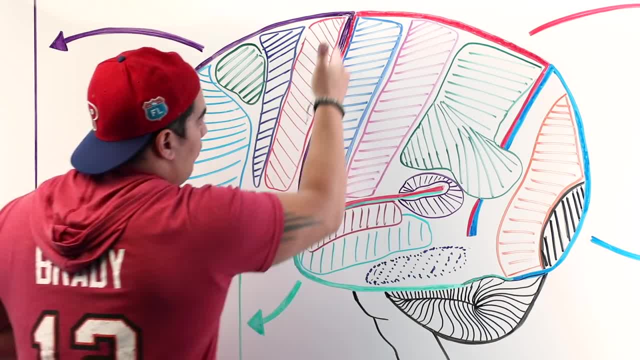 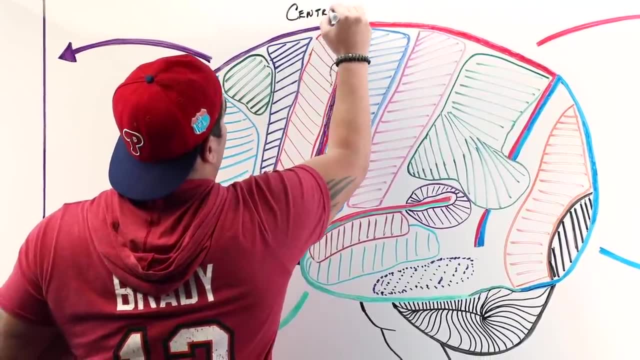 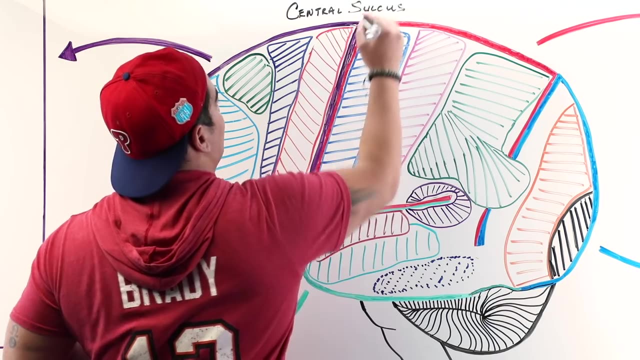 You can kind of see it in a combination of red and purple. It's this one right here. This little sulci here is called your central Sulcus. It's called your central sulcus. Now, your central sulcus is beautifully placed, that it. 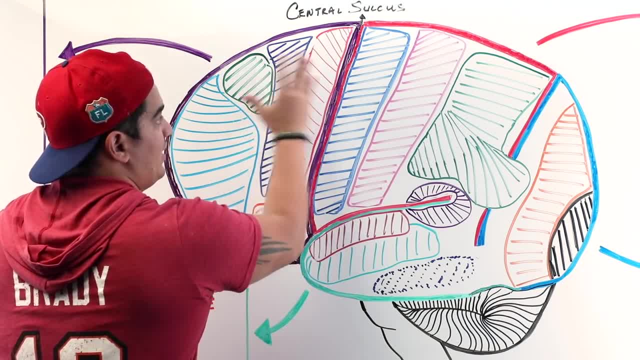 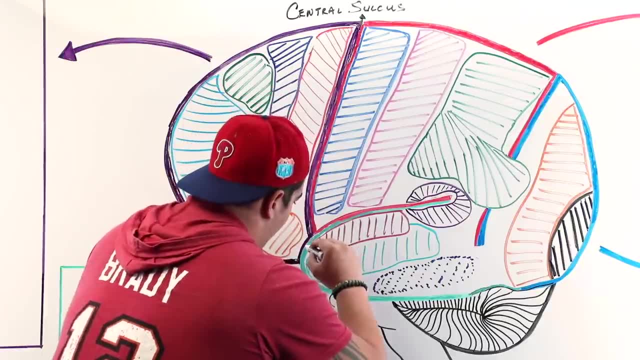 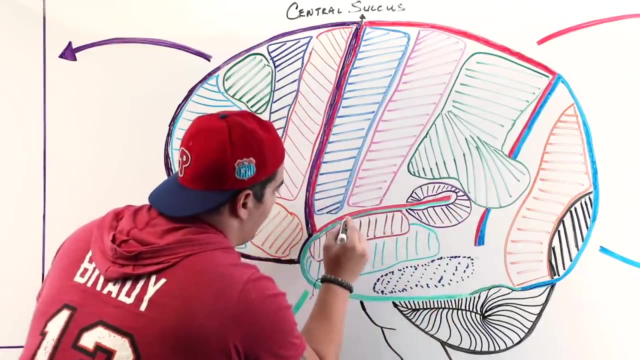 separates what two lobes? Your frontal lobe, which is anterior to it, and your parietal lobe, which is posterior to it. right, There's another sulcus. Another sulcus is running here. right, this color here, So this red and green one here, This one here. I'm going to have a line coming out from it. 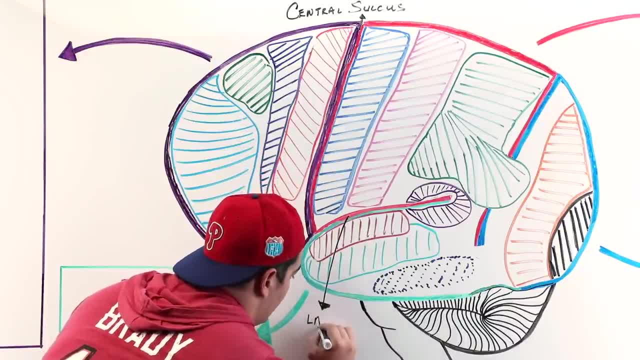 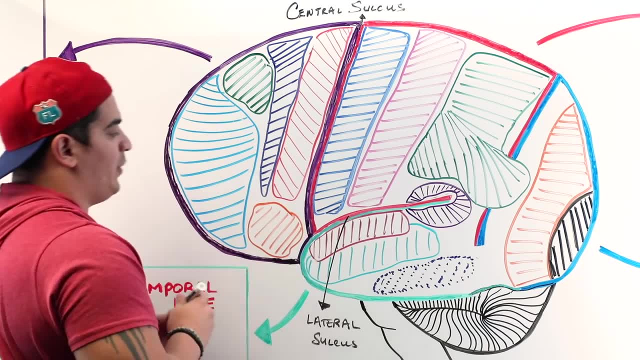 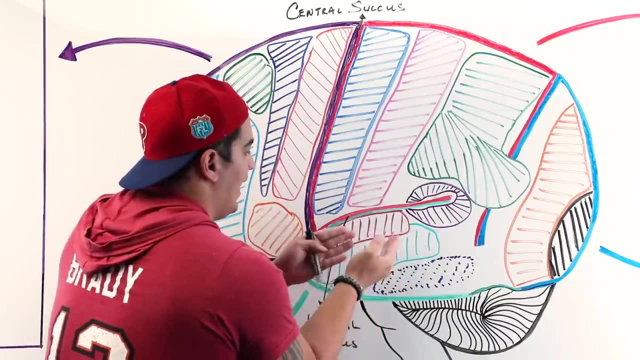 This here is called your lateral Sulcus. It's called your lateral sulcus, Sometimes also referred to as your sylvian fissure. okay Now, the beautiful position of the lateral sulcus is that it separates this lobe, the temporal lobe. 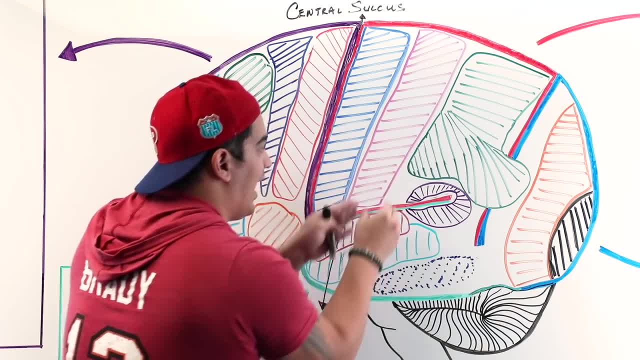 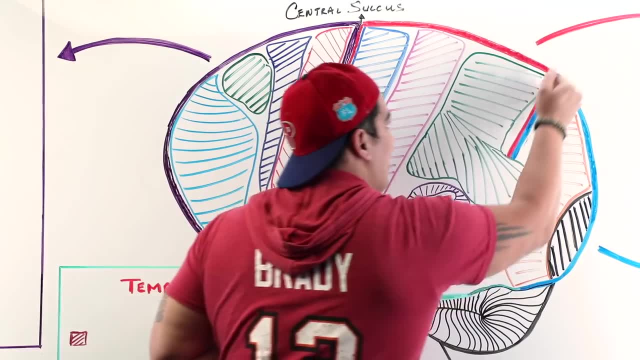 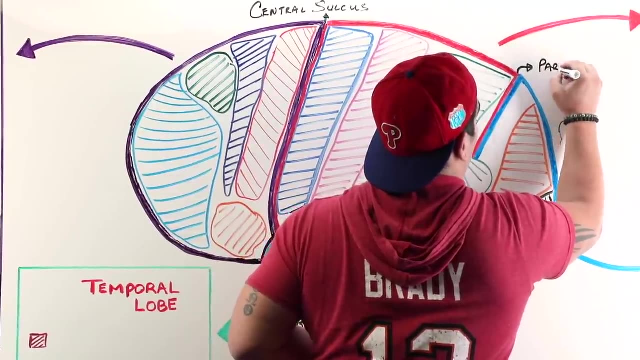 from the frontal lobe and the parietal lobe. okay, That covers that demarcation. There's another demarcation here, right here, This kind of blue and red one here. This guy, This guy is called your parieto-occipital sulcus. 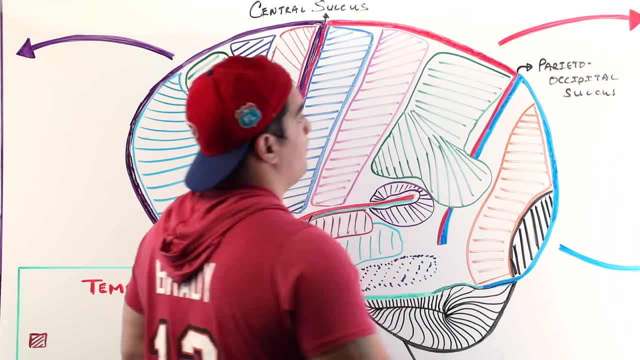 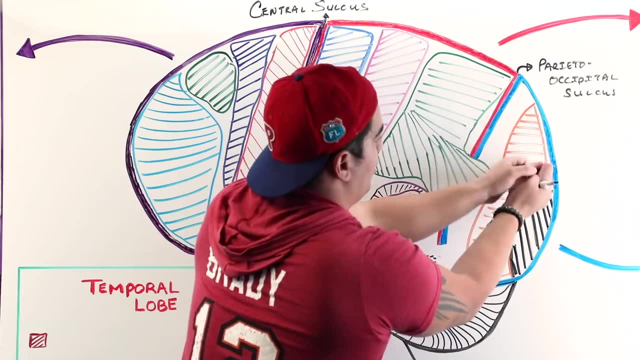 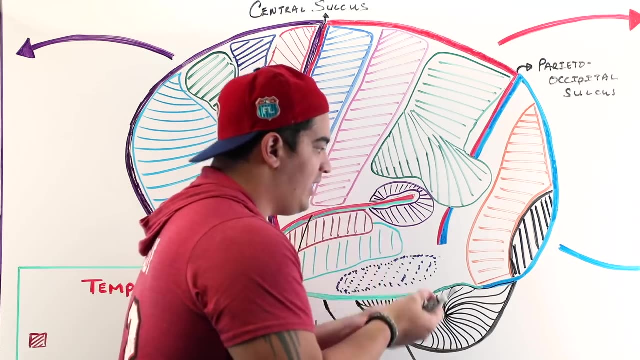 Now, the beauty about the parieto-occipital sulcus is that it's positioned in such a way that it separates, anterior to it, the parietal lobe, from posterior to it, the occipital lobe. okay, Now, this last one here is not a actual complete. 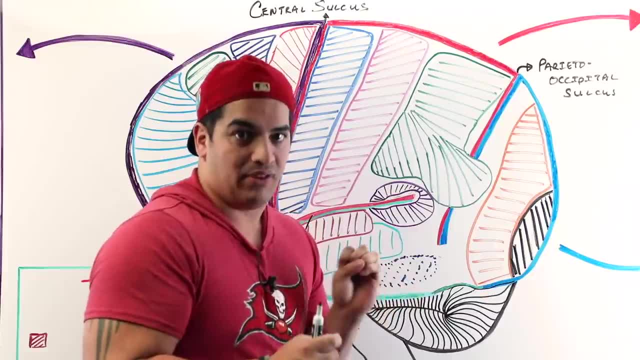 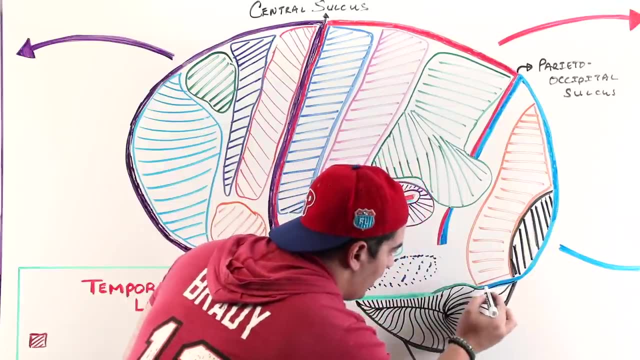 sulcus or demarcation. It's an imaginary type of line. Right here you see how we come from this occipital lobe just above this cerebellum. There's a little notch right here. right here I'm going to kind of draw it here in this dark black. 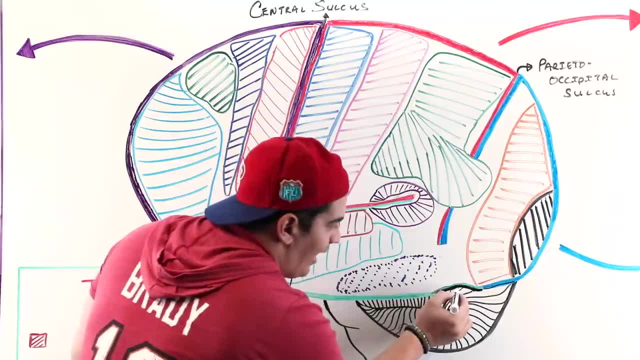 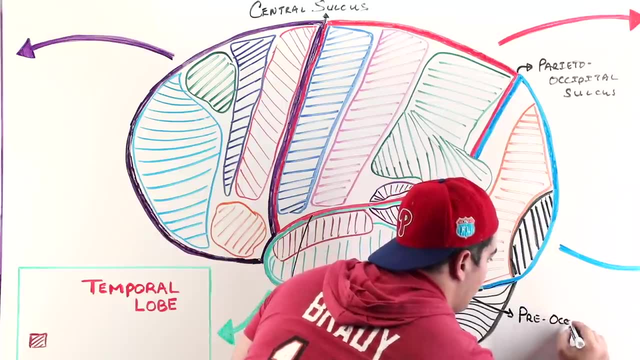 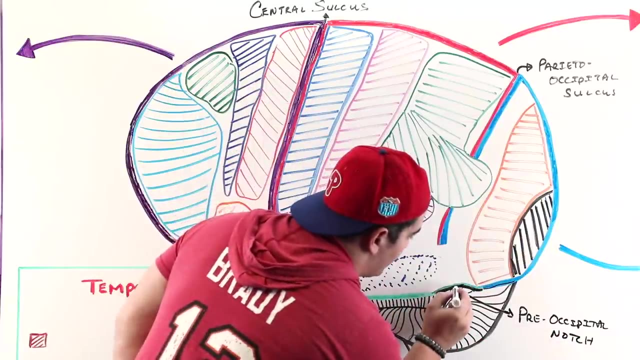 here, right, You see that little notch, that little kind of elevation point, That elevation point right there is actually referred to as the pre-occipital notch, And if you draw an imaginary line from this little notch or this pre-occipital notch towards your parieto-occipital 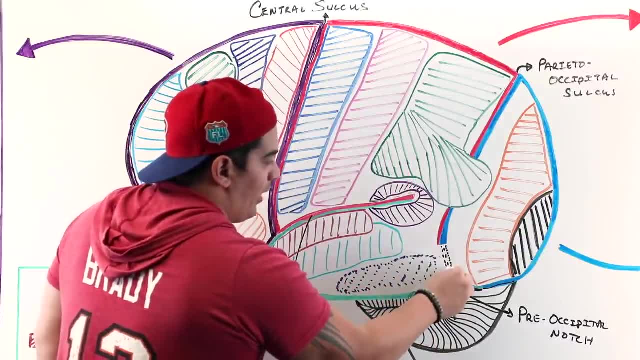 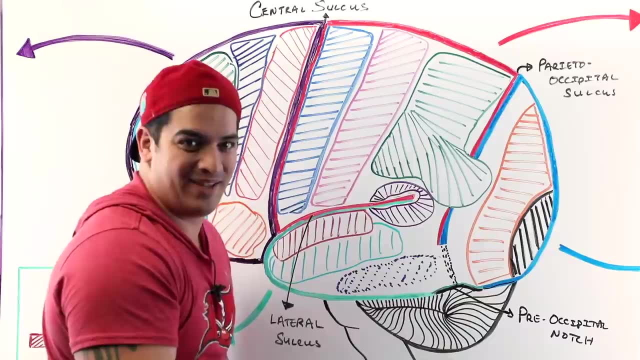 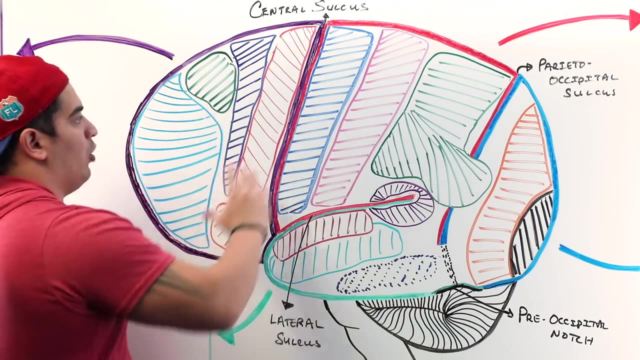 sulcus. Guess what that does? It separates your occipital lobe, which is posterior to it, from your temporal lobe, which is anterior to it. So that is going to give us our demarcations. Now what I want us to do is start here with the frontal lobe. Talk about some of the, the names of these areas, and 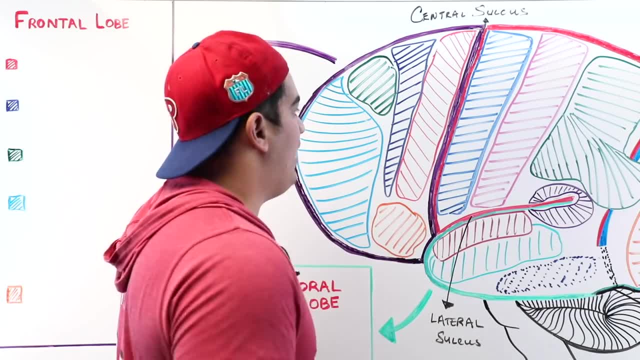 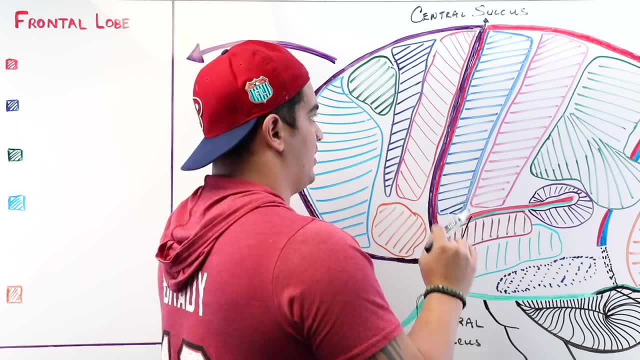 then come over and talk about their basic function. All right, so now what I want us to do is talk about the particular areas. I just want you guys to know where they would be in kind of a general sense. There's no complete clear-cut demarcation. 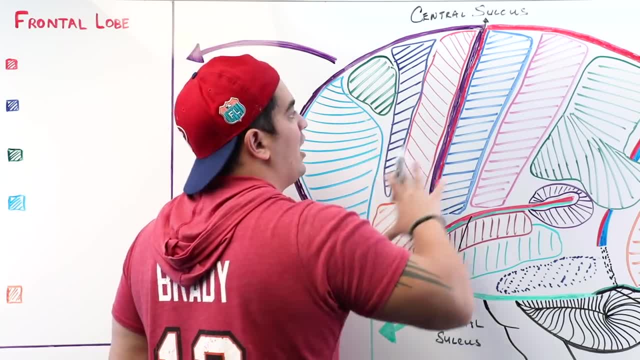 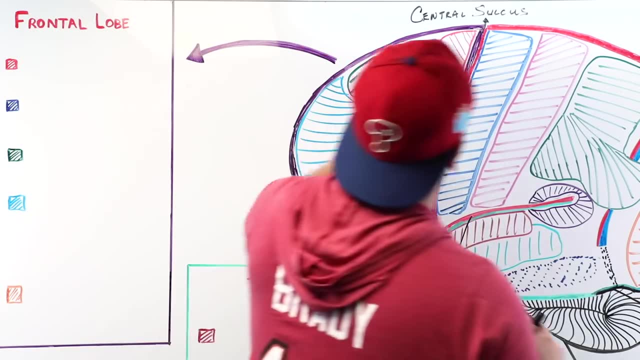 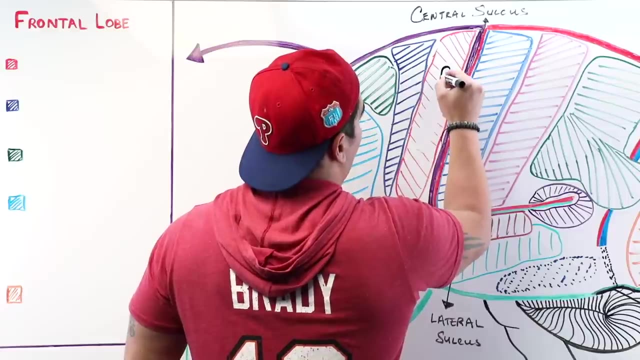 like we have with the central sulcus between each one of these kind of general areas in the frontal lobe. So this first area here, this is very important, this kind of red one here, This area here is very important. It's called your primary motor cortex, But we're just going to abbreviate it for 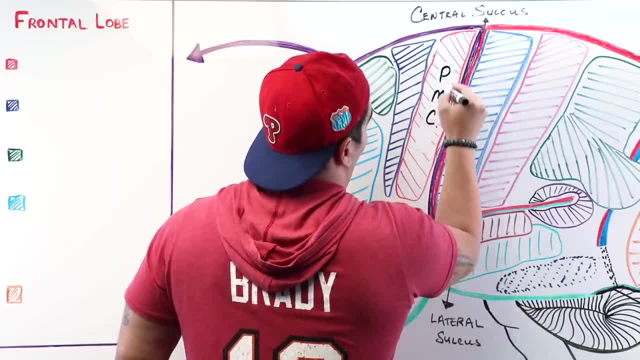 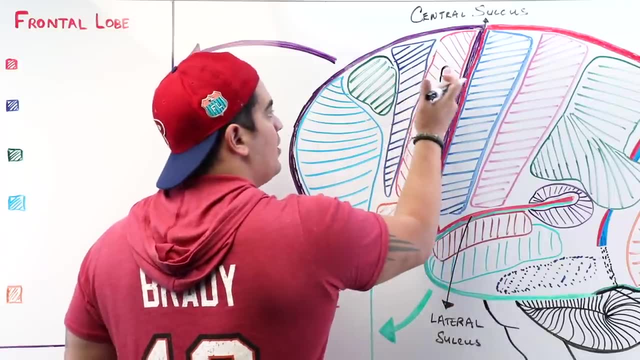 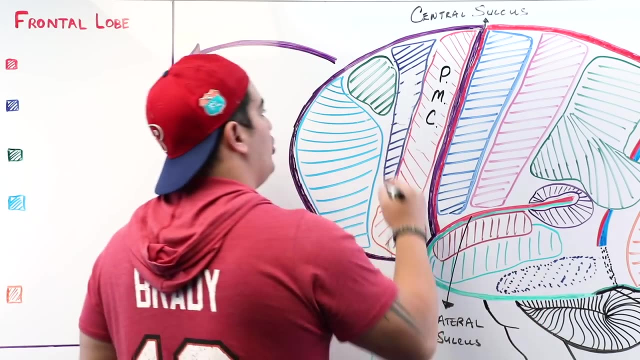 right now as P MC. We'll write it down later. Now, just anterior to that, because I just want you to know the general position in anatomy, Just anterior to the primary motor cortex, you have this blue one here. This blue one here is very important as well. It is called your motor association cortex. It's made. 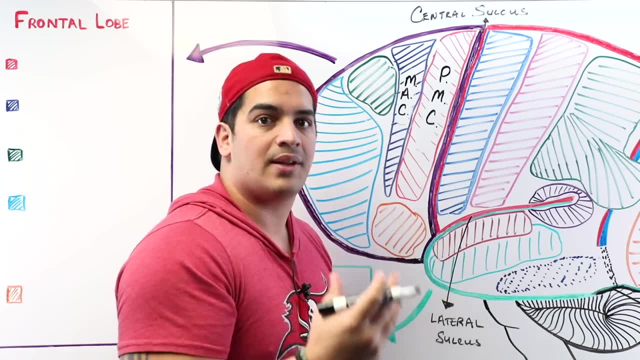 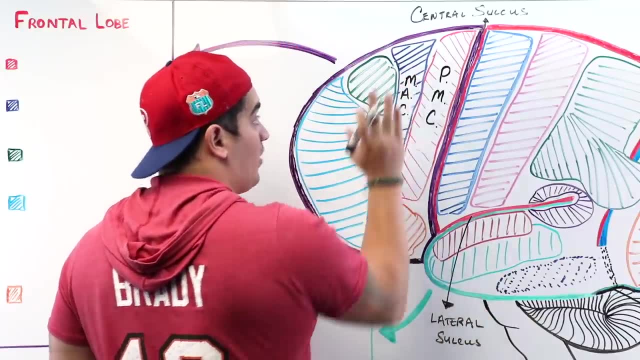 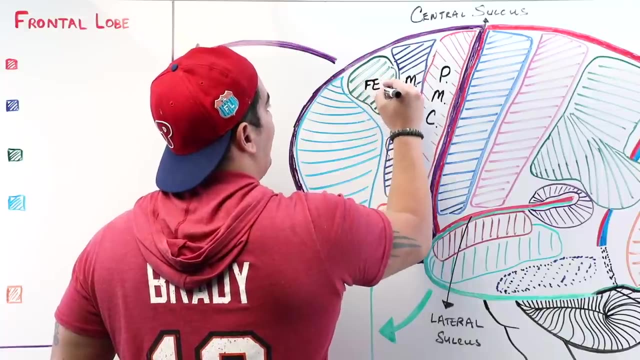 up of two particular areas called the premotor cortex and your supplementary motor cortex. You have a little bit anterior to that, more in the superior aspect of the frontal lobe, You have another area in this green color. This is called your frontal eye fields. Then just go a little bit. 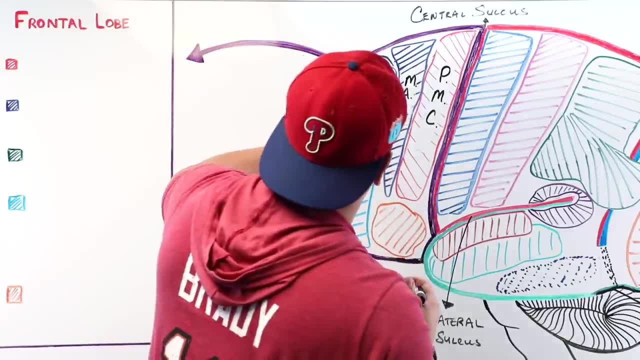 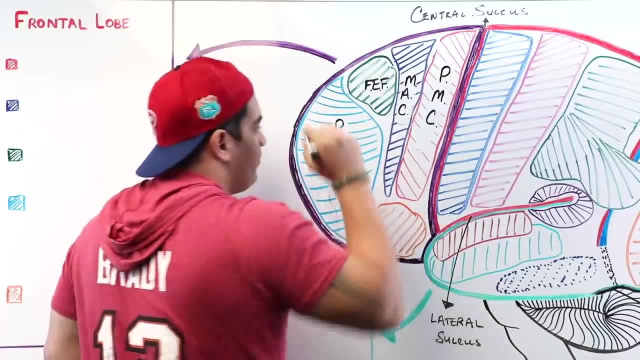 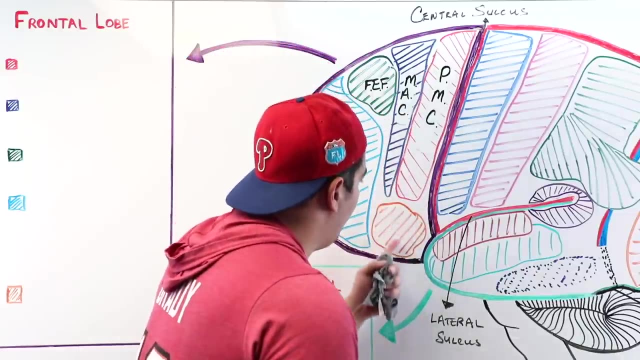 anterior and inferior to the frontal eye fields in the frontal lobe And you got this big blue structure here. This is called your prefrontal cortex, Sometimes also referred to a textbook as the prefrontal association area. You come at the most inferior point of the frontal lobe, usually on the left side of the brie You have 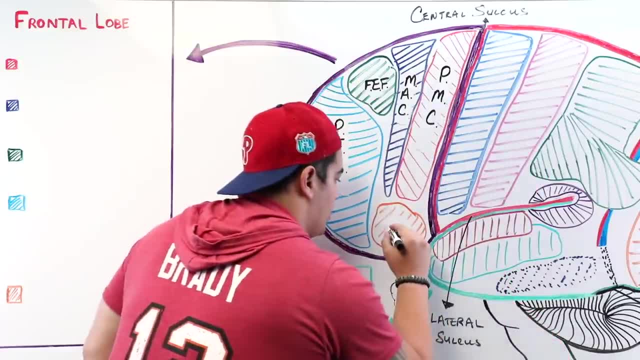 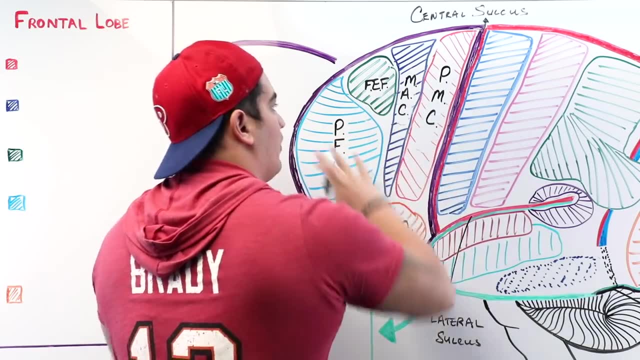 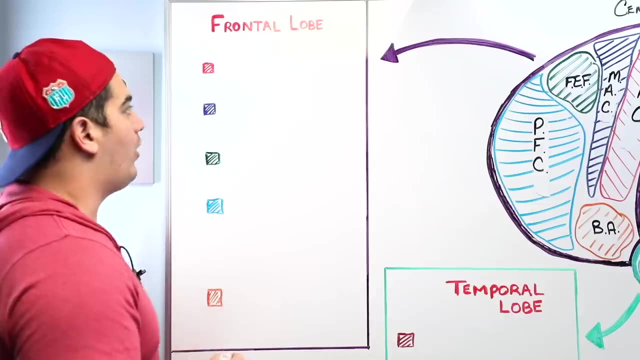 another area here called- and this is in orange- This is called your Broca's area. So this is the general anatomy in the frontal lobe of these particular areas. Now let's come over here into this chart and talk about the general functions of the each of these areas. All right, So we talked. 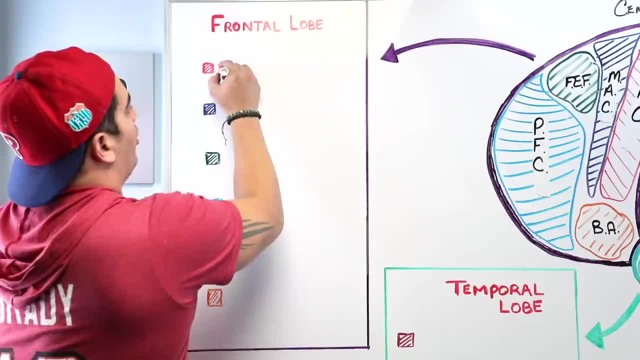 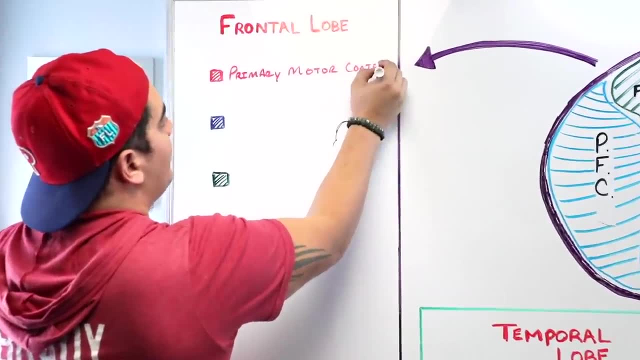 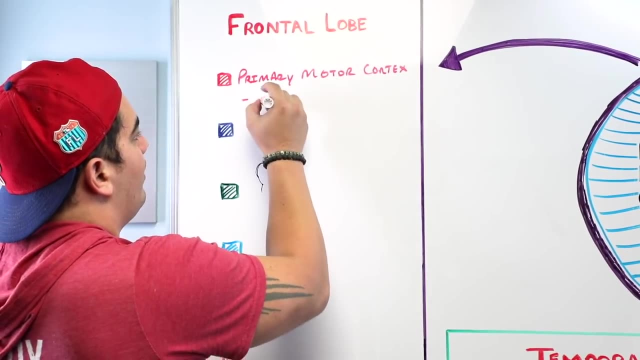 about each one of those areas in the frontal lobe. So we said the first one is called our primary motor cortex, Right? We call that the PMC. Right Now, the basic function I want you to remember for the primary motor cortex- literally kind of a one kind of liner- is that it's involved in voluntary 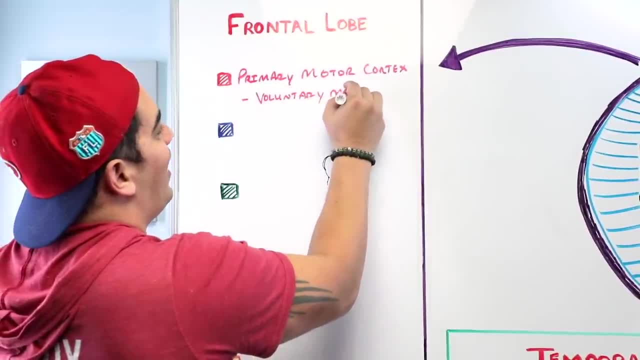 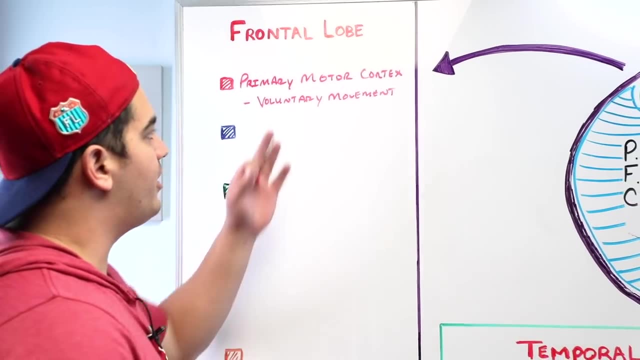 movement. That's all I want you guys to remember. The big thing that I want you to remember, though, as an aside to keep in your brain, is that the primary motor cortex- we're looking at a lateral side of the brain, Right, If we look at the, imagine that this is the lateral side of the brain. 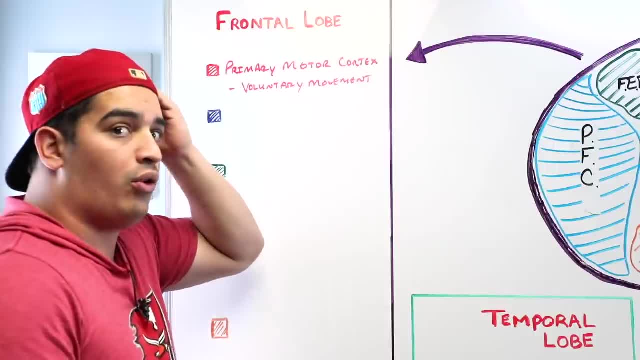 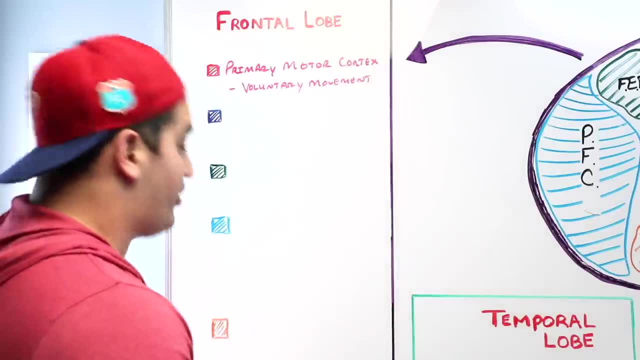 The left side of the lateral surface of the brain, The left primary motor cortex controls movement of your right side. So when I say voluntary movement, I want you to remember that it's contralateral sides. That's all I want you to remember for right now. for the primary motor, 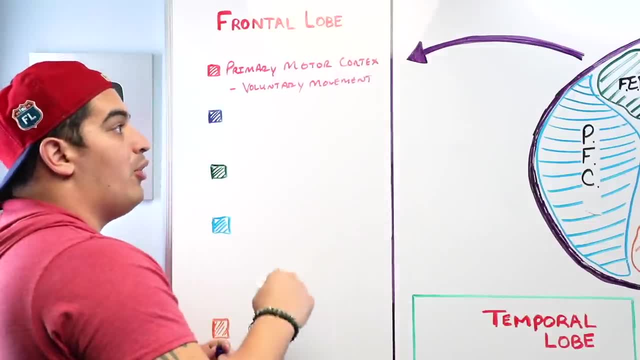 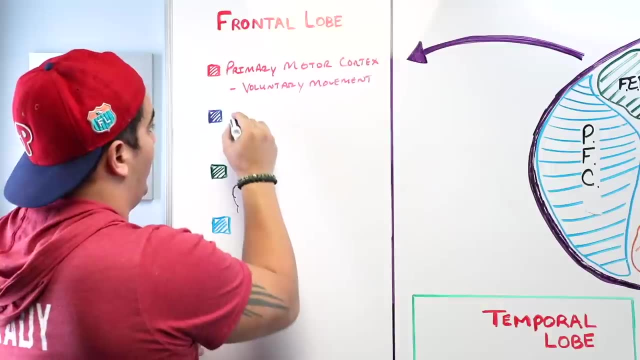 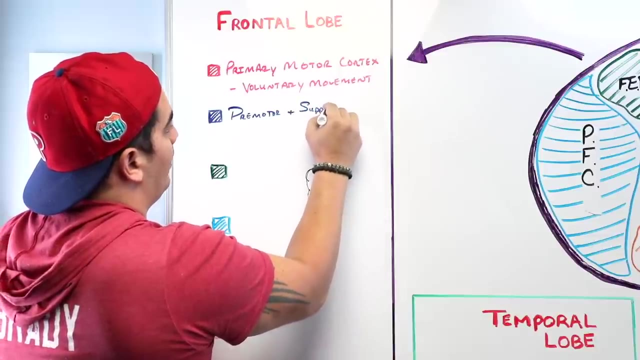 cortex We said just anterior to that was your motor association cortex. Right Now your motor association cortex. I want you to remember that it's made up of two areas- Right, We're going to write them now as your premotor cortex and supplementary motor cortex, Right? So this is. 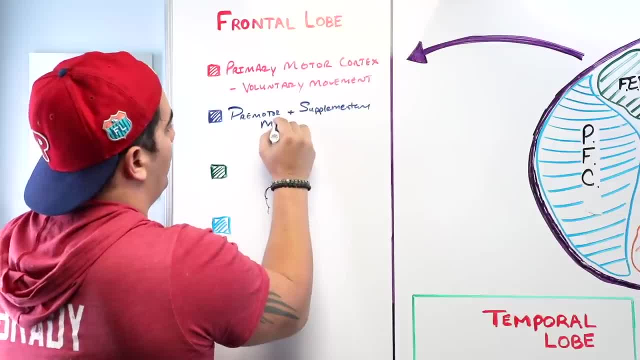 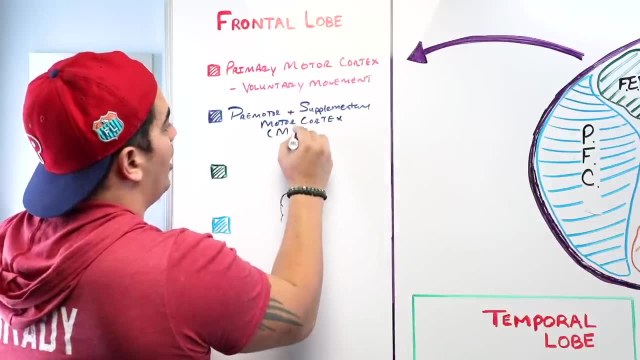 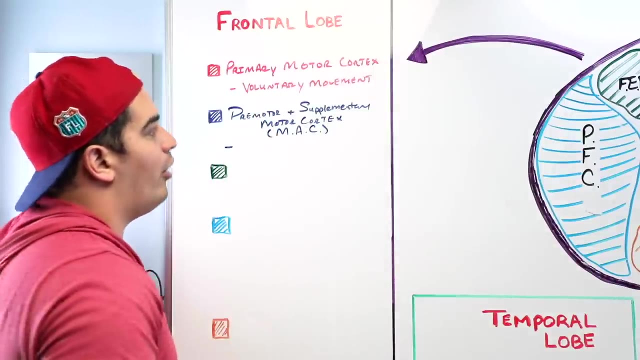 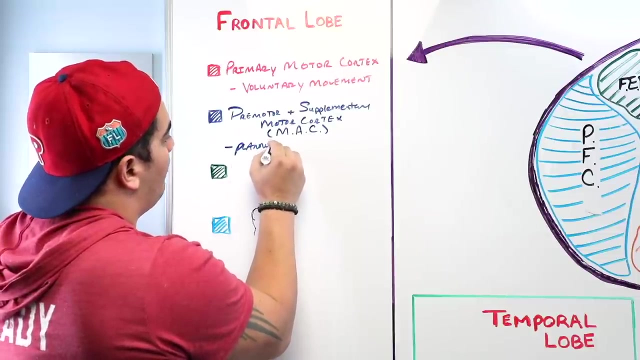 supplementary motor cortex, But again, the combination of these two is called your motor association cortex, Now the premotor and supplementary motor cortex. they also are involved in voluntary movement, But more specifically they're involved in the planning of movement. They're involved in the sequencing of movement, They're involved in the 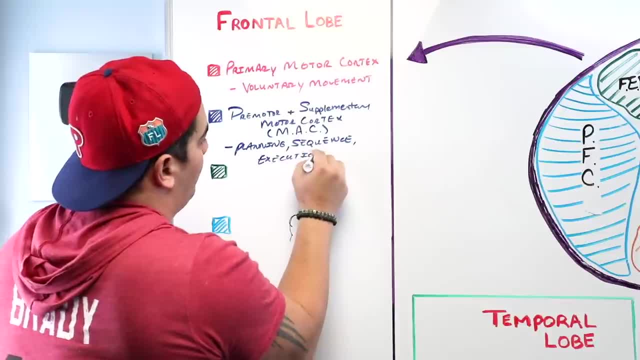 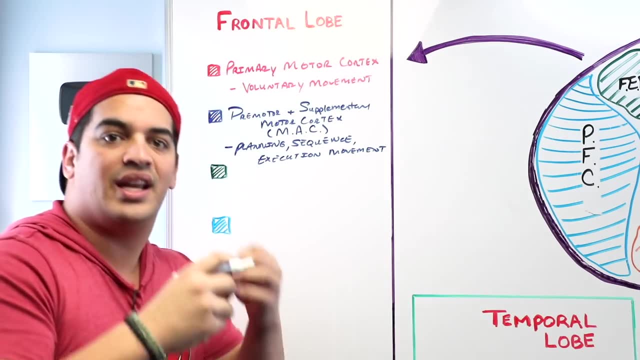 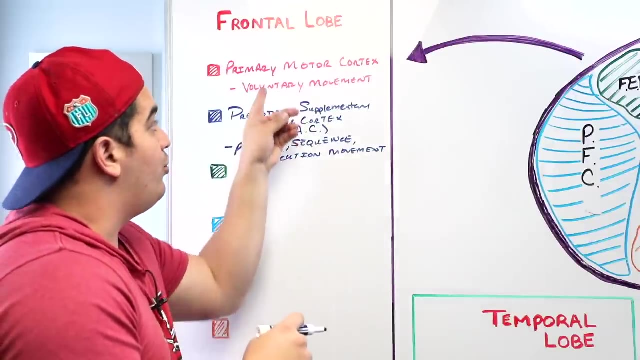 execution of movement Right. So when we talk about how they're involved in movement more specifically, they're involved in the planning, the sequencing and the execution of movement Right. But they do also give some axons from them that do go into the descending motor pathways. 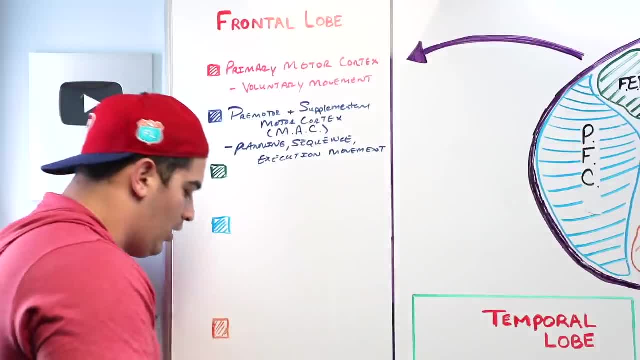 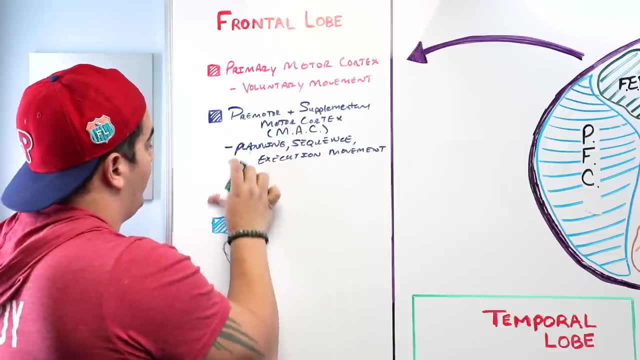 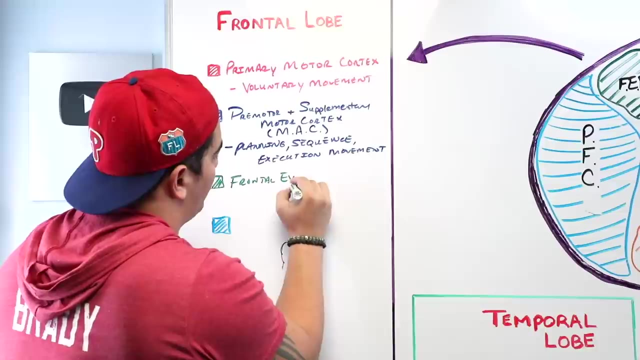 that are involved in movement as well. Okay, The next area just anterior to the motor association cortex is called your frontal eye field. What is it called Your frontal eye field? Your frontal eye fields are also very interesting. They're involved in a kind of a specialized motor movement, And these more specifically: 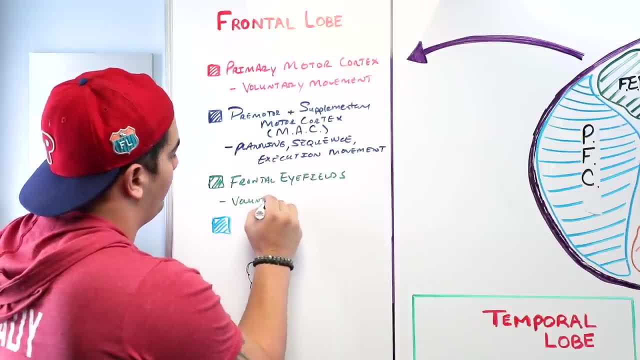 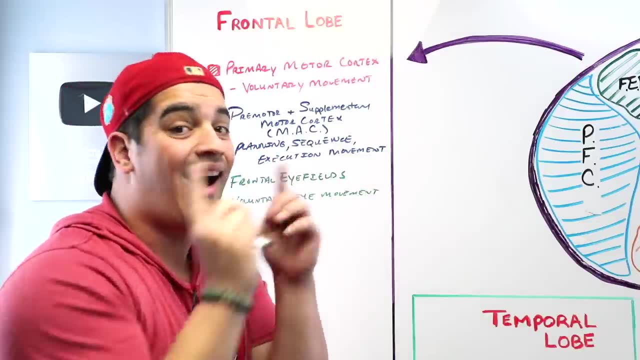 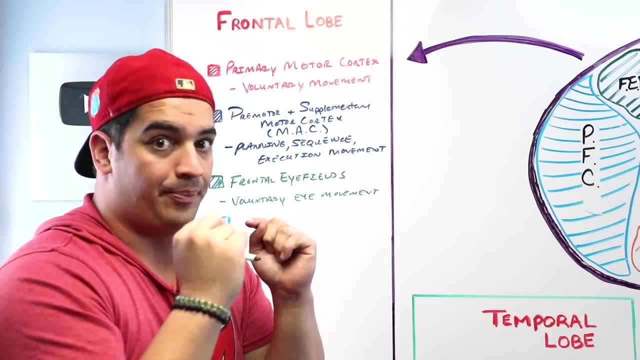 are involved in voluntary eye movement. Okay, If we were to kind of add on to that, it's more involved in what's called saccades, which is rapid eye movement, So helping your eyes to move conjugately to the left, conjugately to the right, up and down. 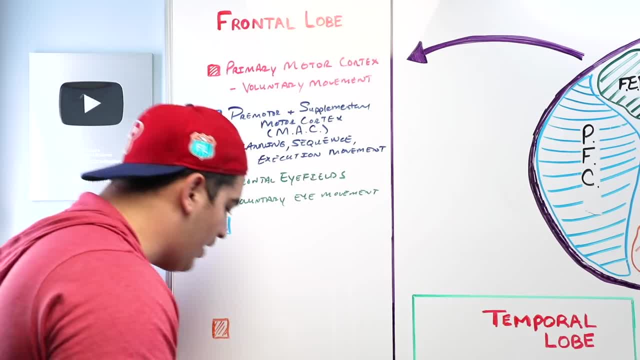 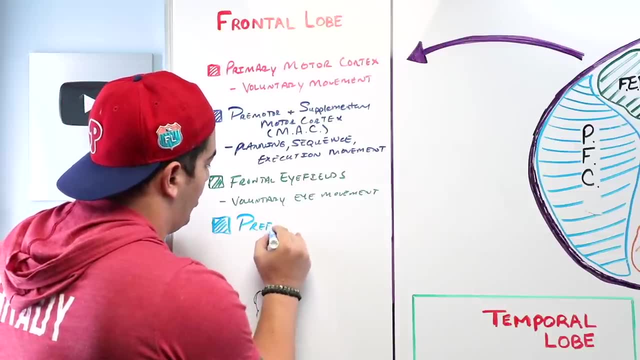 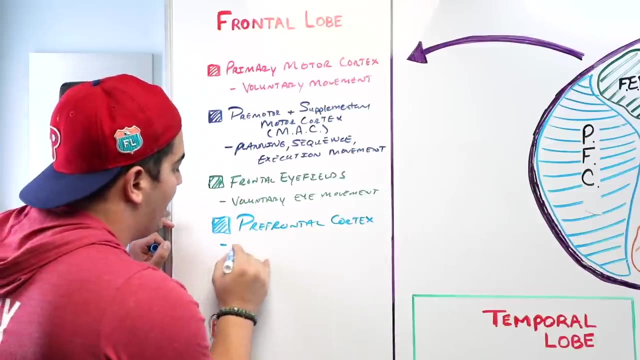 Okay, So that's your frontal eye fields. The next one is: if we move just a little bit anterior to the frontal eye fields, we have that prefrontal cortex, So it's called the prefrontal cortex. Now, the prefrontal cortex has so many functions, Right, It's involved. 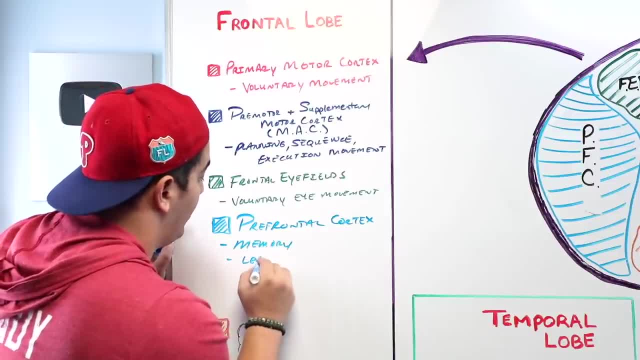 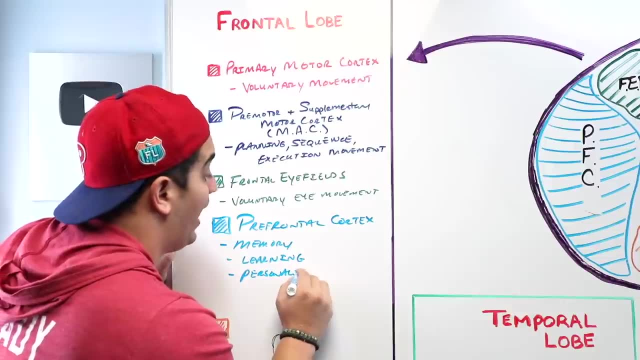 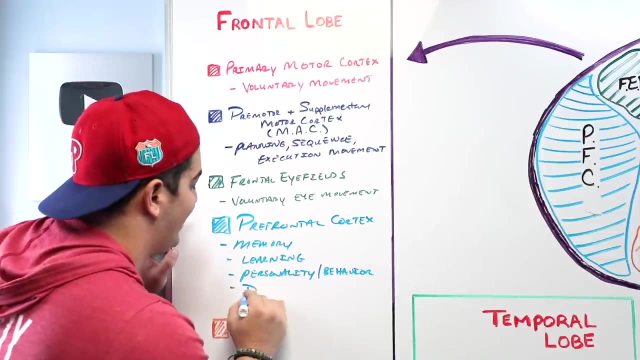 in our memory. It's also involved in learning, So kind of in the cognition process as well. It's involved in our personality, Right And even our behavior, And it is also involved in our judgment, our reasoning or kind of we can say decision making. 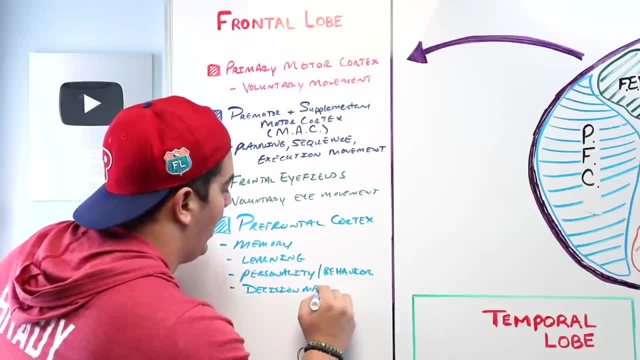 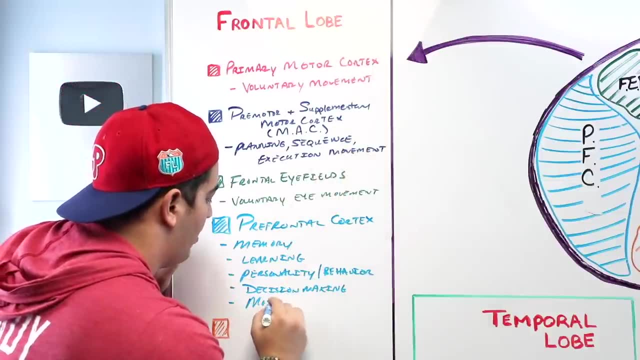 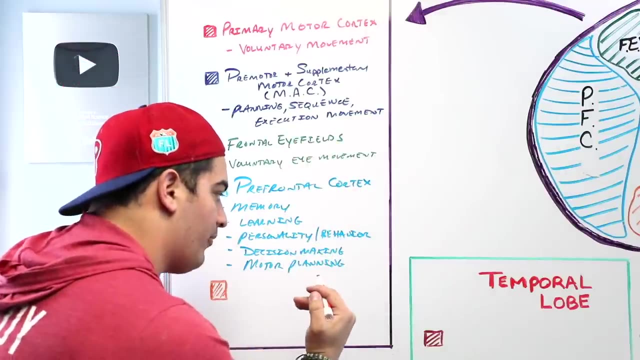 Right, So it's also involved in our decision making And, last but not least, it even has some type of input that it can send to your motor association cortex that is involved in motor planning. All right, In the last area, that orange area that we said is usually like the bottom of 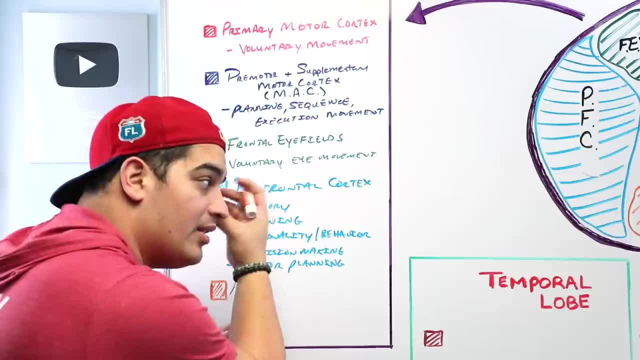 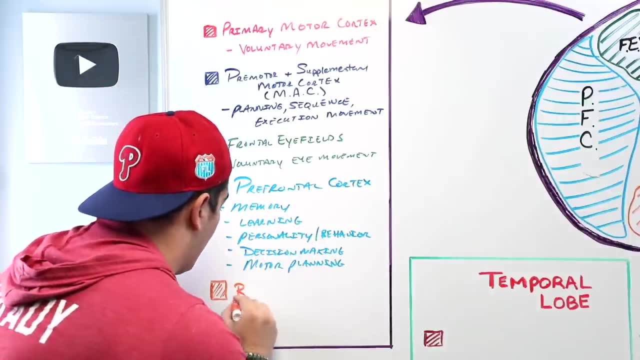 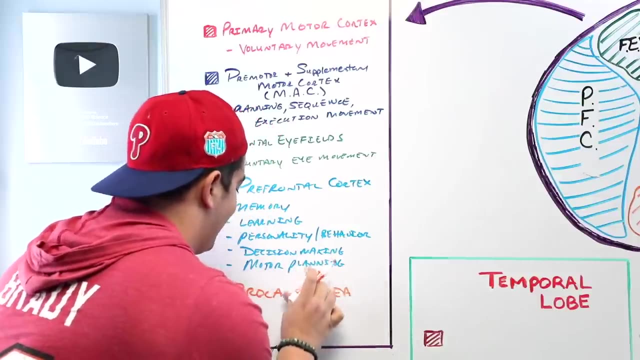 the frontal lobe, Usually the most inferior portion, more commonly on the dominant side of individuals, The cerebral hemisphere which is usually their left because they're most likely right handed dominant, is your Broca's area. Okay, So Broca's area Now, Broca's area is important because it's involved with our speech. 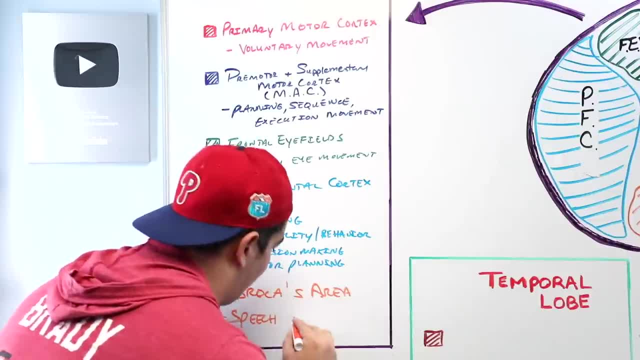 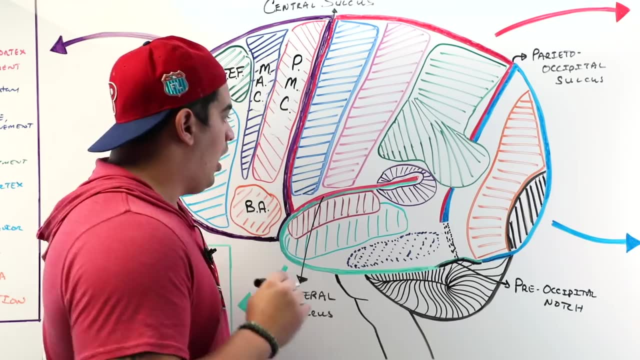 production, So it's involved in stimulating the muscles that are involved in speech production. All right, Beautiful. So that covers our Broca's area. Now let's talk about the areas of the temporal lobe and their function. All right, Great. So we talked about the frontal lobe. We went over. 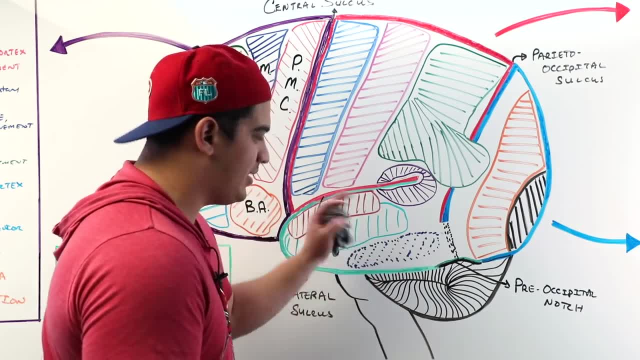 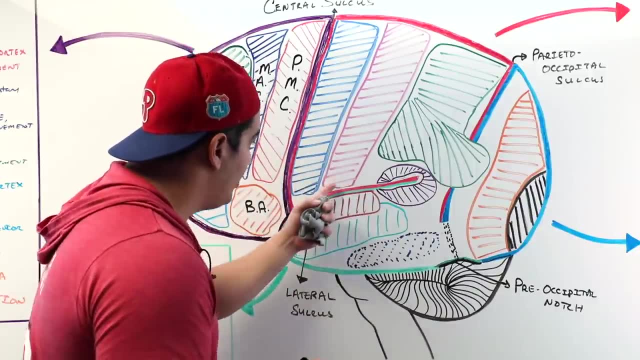 the areas, their functions. Now let's talk about the temporal lobe. These are areas, basic anatomy and then functions. All right, Remember we had that lateral sulcus Right, So that's separating our temporal from our frontal and parietal just underneath the lateral. 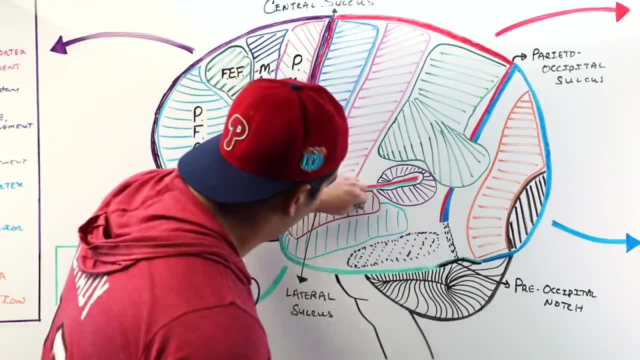 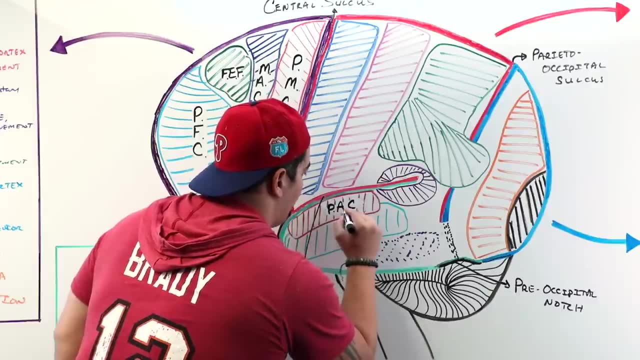 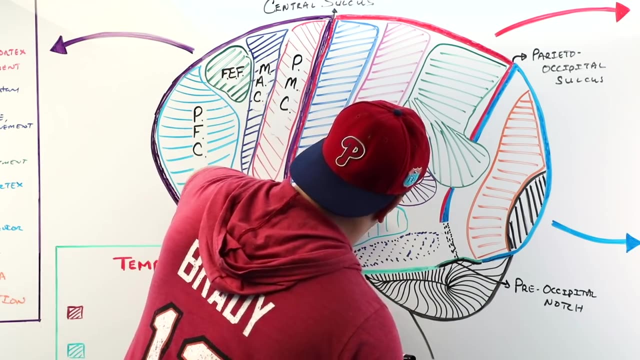 sulcus. You have this kind of like red area here, Right, This red area here is very important and it's involved in sound. This is called our primary auditory cortex. Okay, Just below that, Okay, Surrounding it, is another area in this baby blue color And again it's inferior to it. 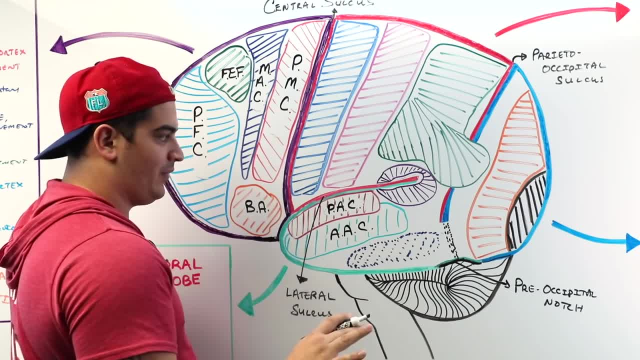 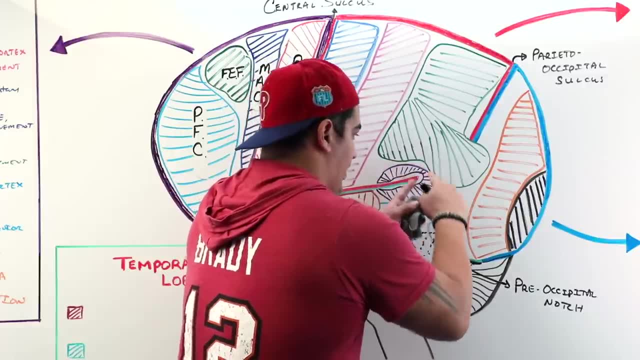 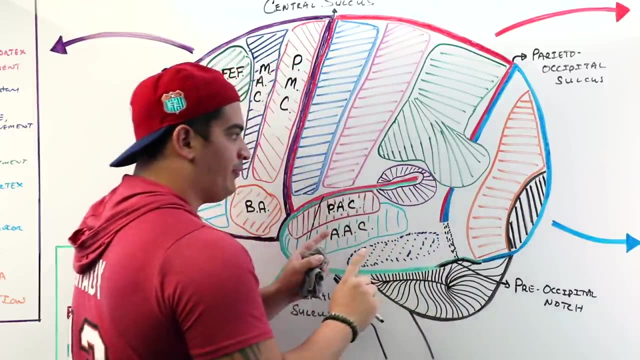 auditory association cortex. okay, The other area here. if we follow lateral sulcus backwards, you have this purple area here And if you look, it's in the temporal lobe mainly, but a little bit of it dips over into the parietal lobe. okay, This area is called Wernicke's area And just like. 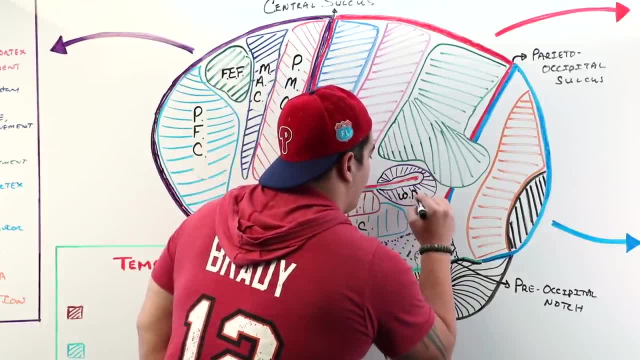 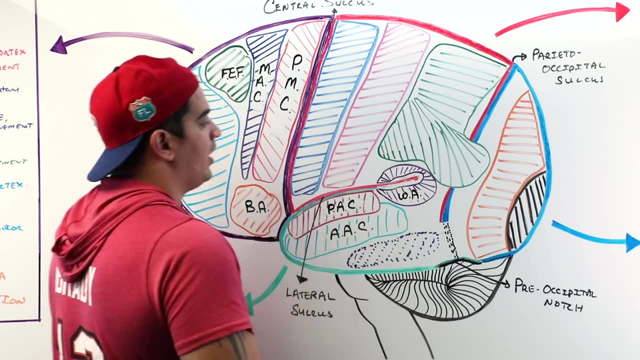 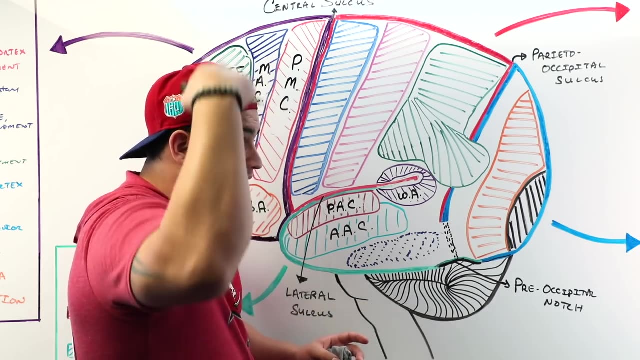 Broca's area. it's primarily only found in the dominant cerebral hemisphere, So usually the left side of the brain for more commonly right-handed people. Now, this other area, this is a lateral surface of the brain. So you're looking at the brain, your eyes are here, you're looking at the 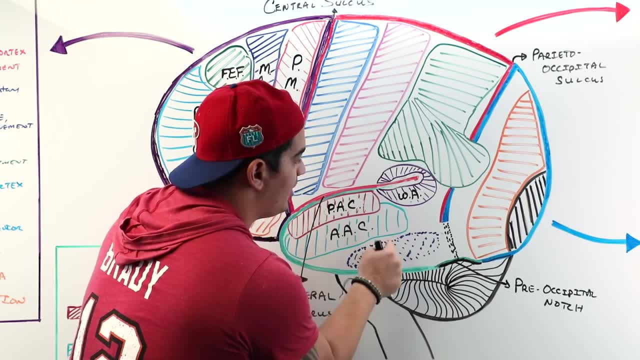 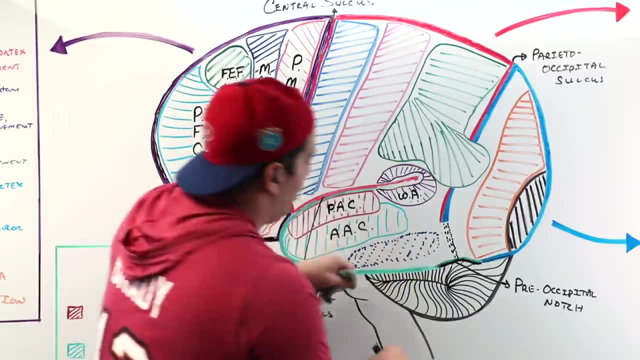 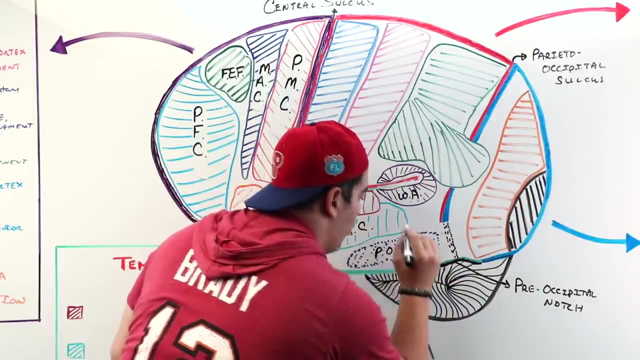 lateral surface of the brain. okay, There's an area in the temporal lobe- but it's deep, It's medial, It's in the most medial aspect of the temporal lobe- I'll show you a picture a little bit later, But it is right here- called the primary olfactory cortex, And there is an association. 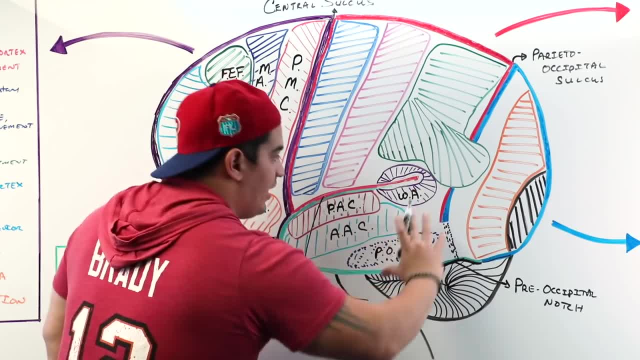 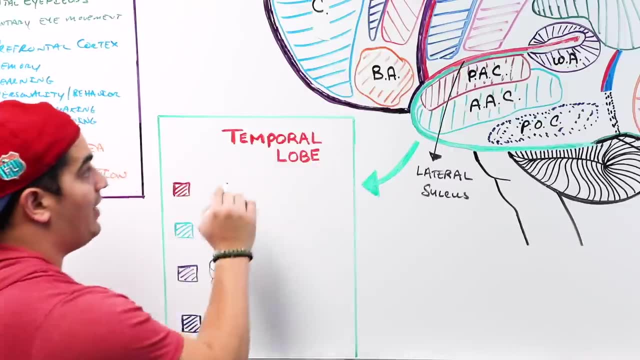 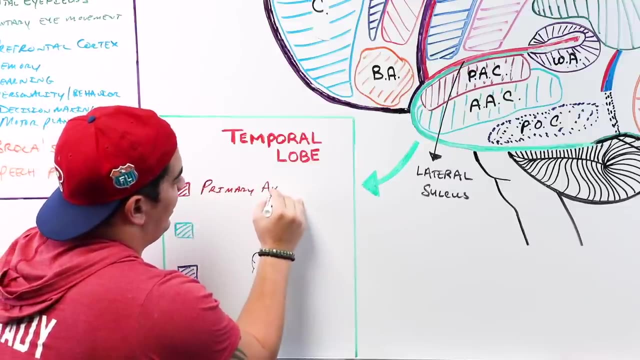 cortex along with that. okay, So these are the areas of the temporal lobe. Now let's talk about their functions. All right, so temporal lobe. Again, we said that we had that first area there just underneath that lateral sulcus. there was called our primary auditory cortex. Now 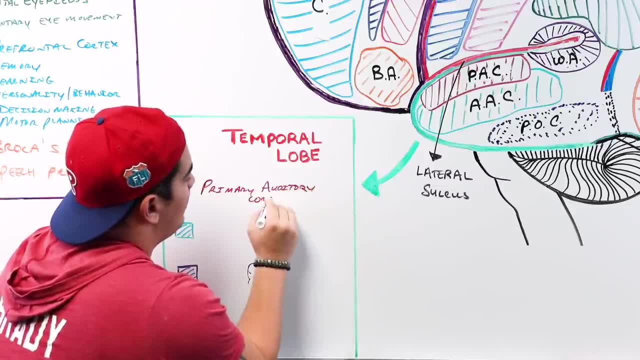 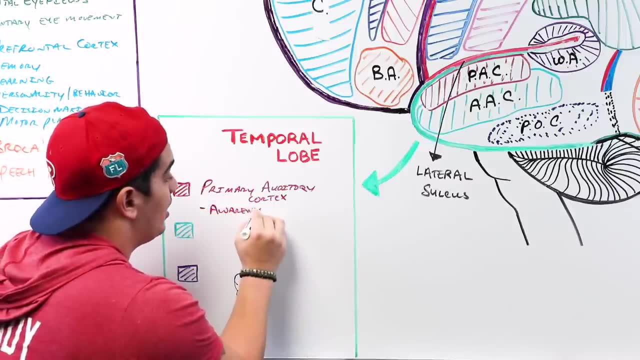 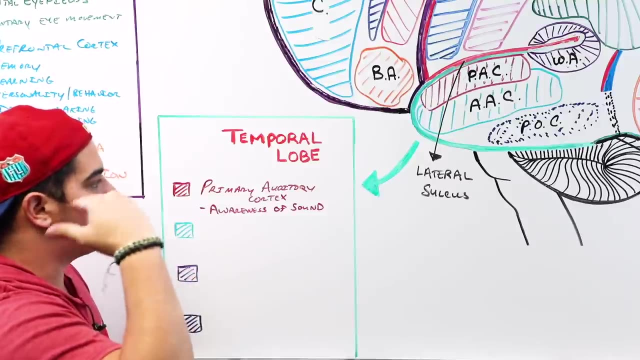 this primary auditory cortex is very cool. It's involved with the perception of sound, right. So basically being aware that we're hearing something. So awareness, consciously conscious awareness of sound. But here's the cool thing, Whenever sound waves basically are carried in the air and then 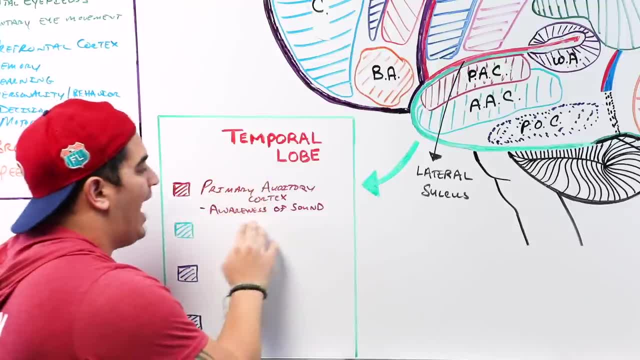 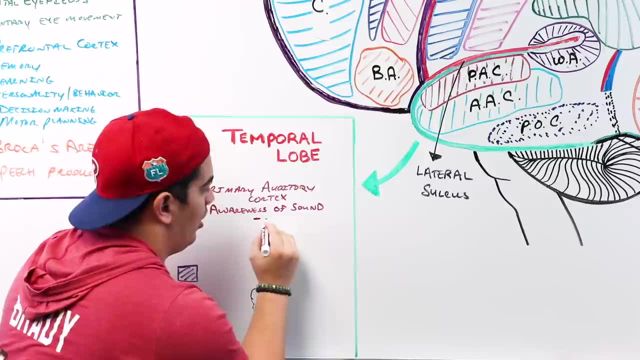 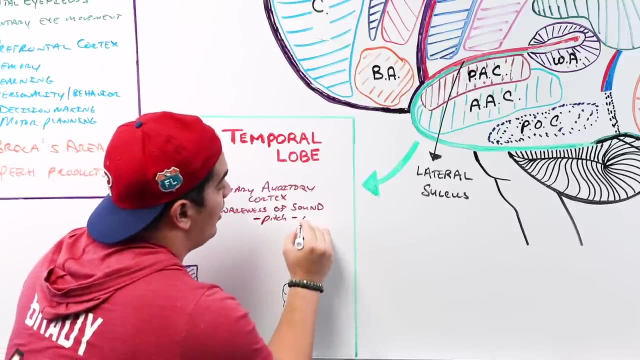 into our ear and then sent to our brain their actual sound waves. our primary auditory cortex really only responds to a couple aspects of sound: The pitch of sound. right, It also responds not just to the pitch of sound but also to the frequency of sound, And it even can determine. 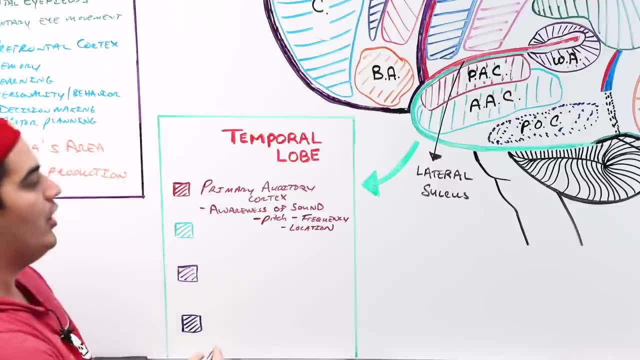 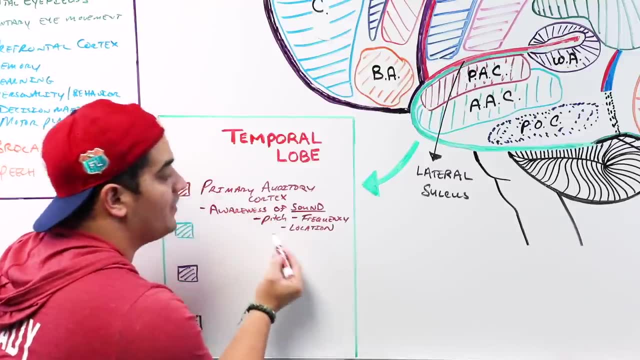 the location of sound, So it can even localize sound. So when we're referring to sound, the primary auditory cortex is involved with conscious awareness of the pitch of sound, frequency of sound and location of sound. Now the other area which we said is just below, it is called 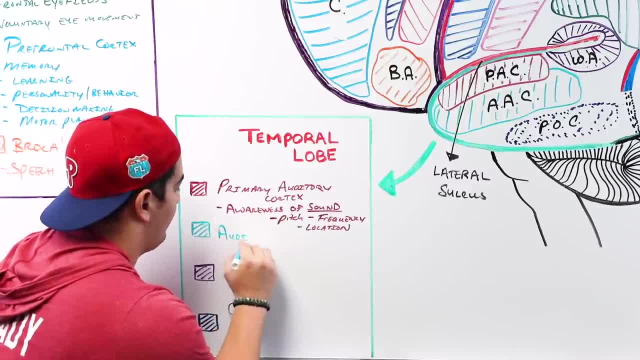 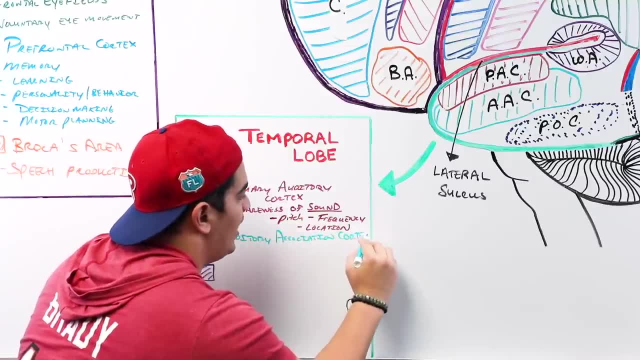 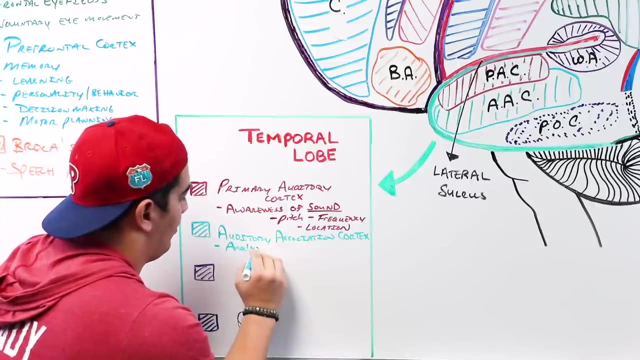 the auditory association cortex. It's called the auditory association cortex Now. the auditory association cortex analyzes the sound. So when we're referring to sound, we're referring to the sound right. So one of the functions here is that it analyzes the sound right. So it analyzes the. 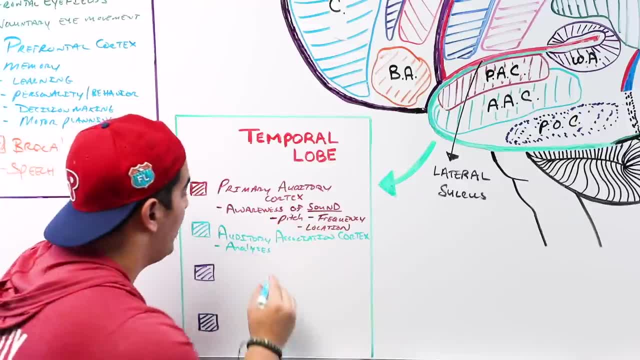 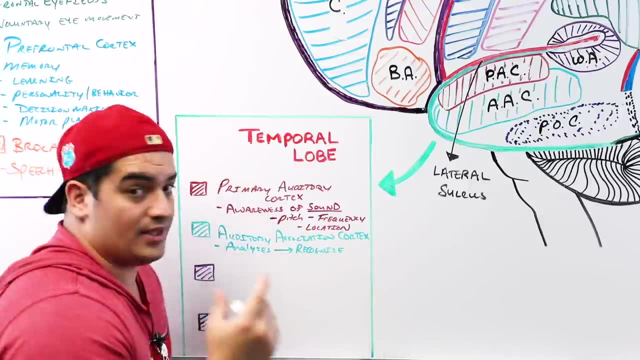 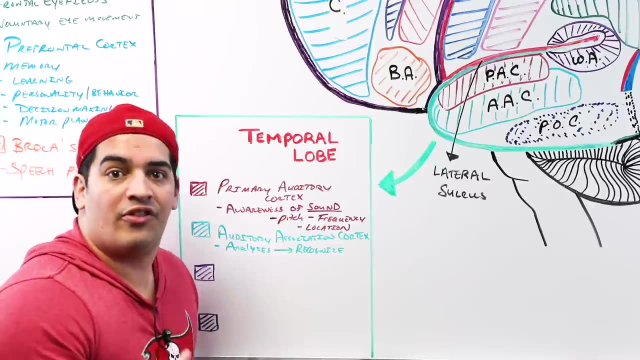 pitch, the frequency, the location, the amplitude, the tone of it, And then, after it analyzes it, it helps us to recognize the sound, what that sound is. Is it someone's voice? Is it a voice that we've actually heard before? Is it even a voice at all? Is it maybe the sound of thunder? 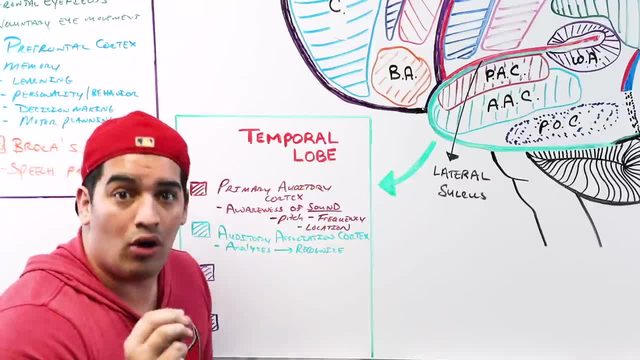 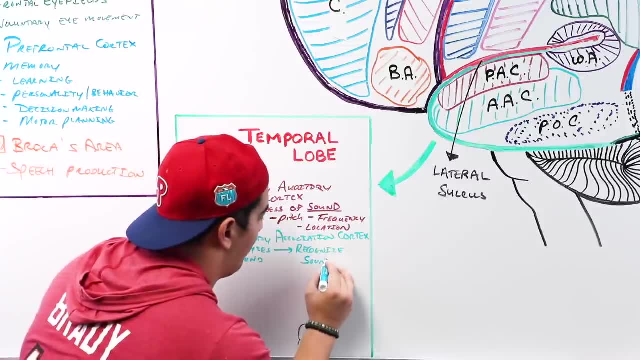 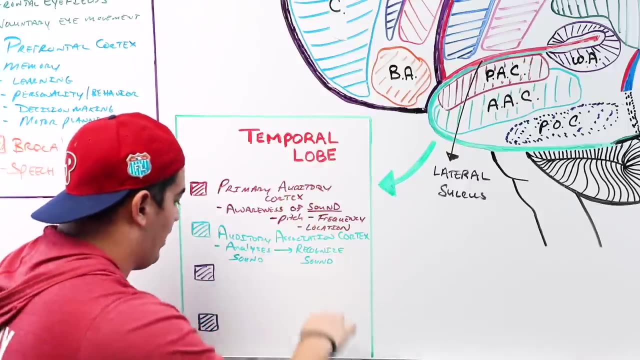 lightning right, All of those aspects it's involved in. okay, It analyzes the sound and it helps us to recognize the sound and store it in our memory. So if we're experiencing that sound again, we'll remember it. The other area which we said is kind of 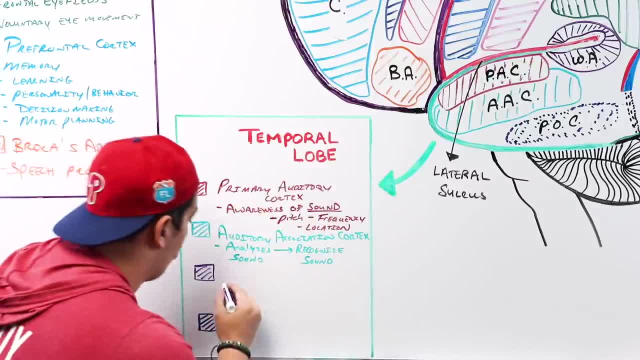 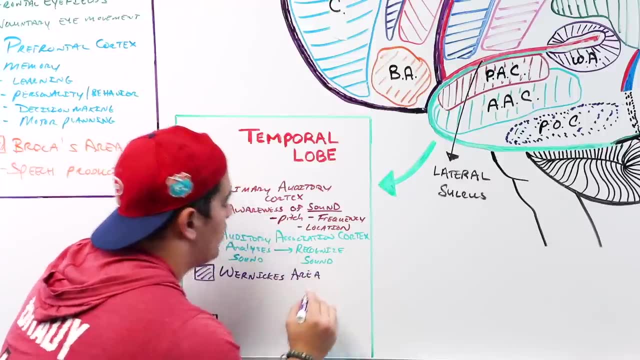 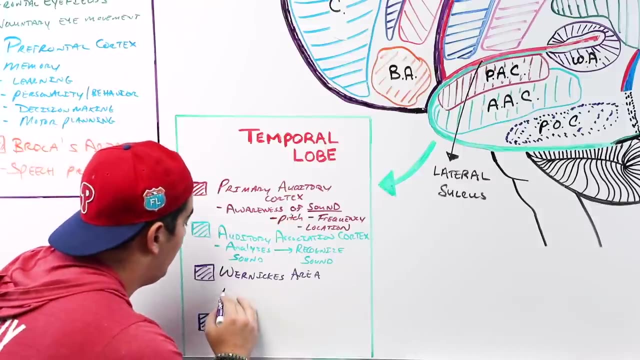 dipping into the temporal lobe and a little bit into the parietal lobe, is called the Wernicke's area. Now, the Wernicke's area is a very cool area that's involved with what's called comprehension and understanding of written and spoken language. So it's involved in 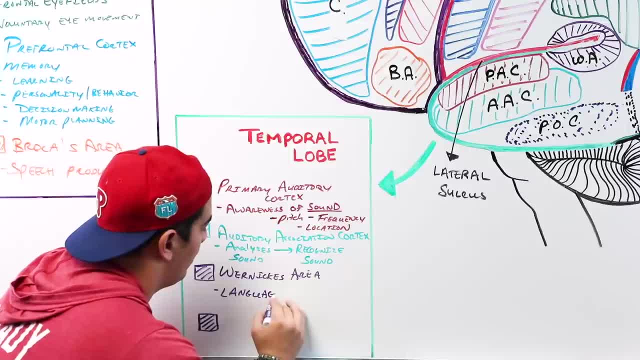 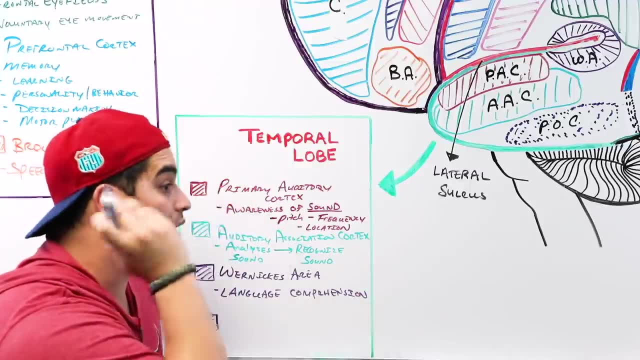 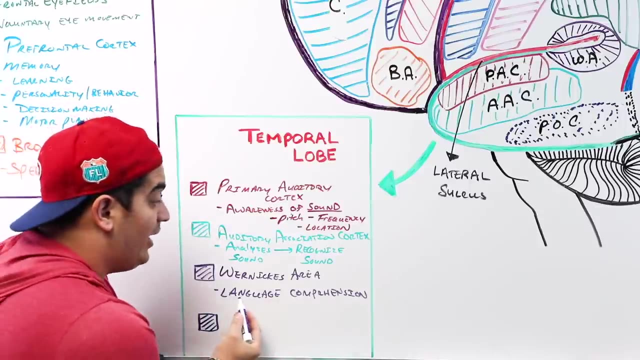 we're just going to say here language comprehension. But again, remember that language can be both spoken, so auditory, we hear it, that language, English language, what I'm speaking to you guys right now and you're hearing through the computer and the written language, me just. 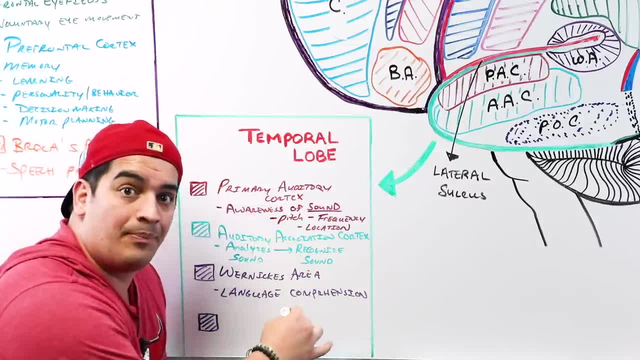 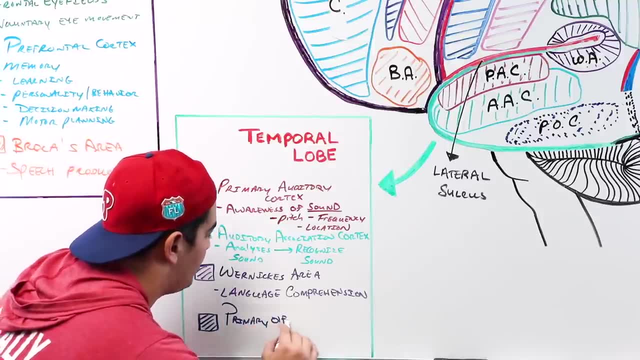 writing down language comprehension. You guys were able to read that. All right. the last area is called that primary olfactory cortex. Now again, I want you to remember that this is not just the primary olfactory cortex, it's the primary olfactory cortex. It's the primary olfactory cortex. 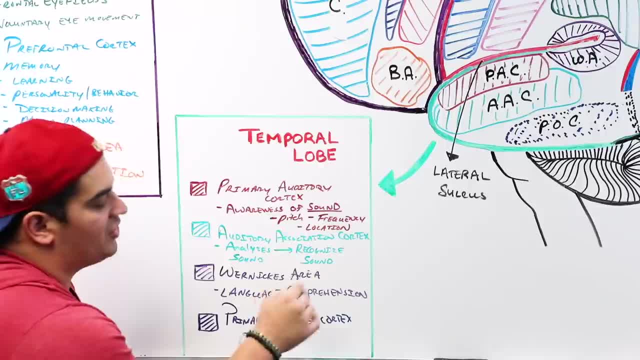 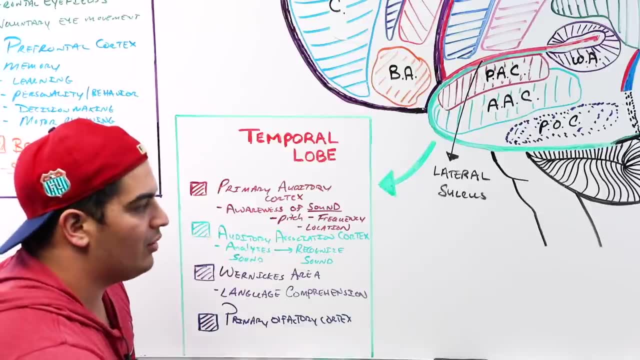 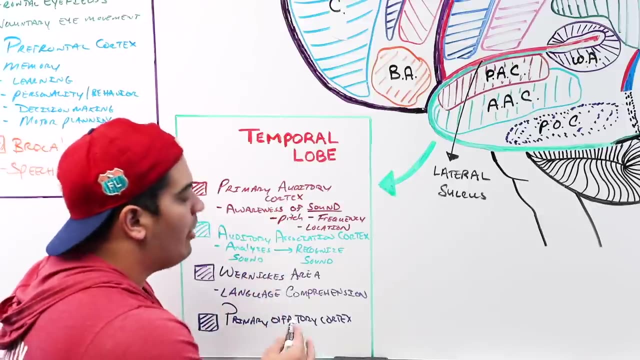 But it also just around that primary olfactory cortex it'll also have an association cortex. Every primary cortex should have an association cortex to analyze and recognize whatever that thing that it's involved in, In this case smell. So to give you guys a little bit more perspective, 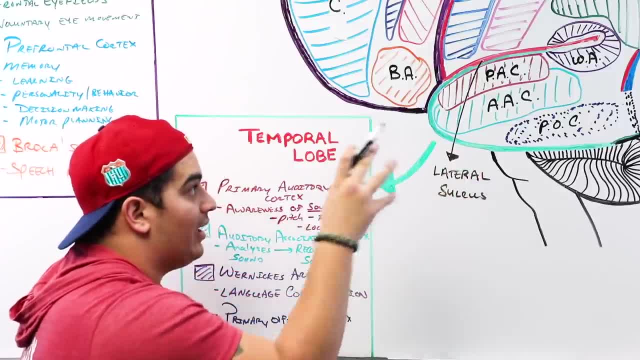 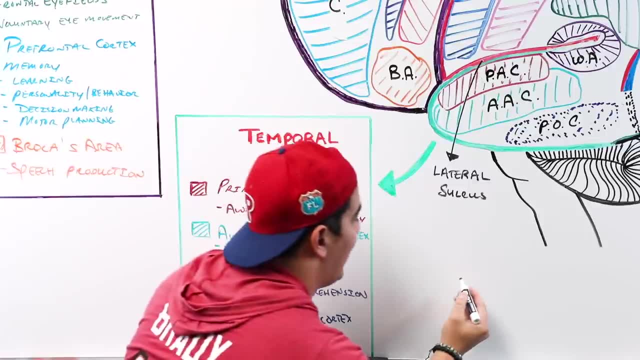 on kind of where, because again, primary olfactory cortex is not on the lateral surface and it's not the most inferior. I just wanted to fit it in there. But if we take again a slice of the brain and we look at the medial surface, you'd kind of see it like this: 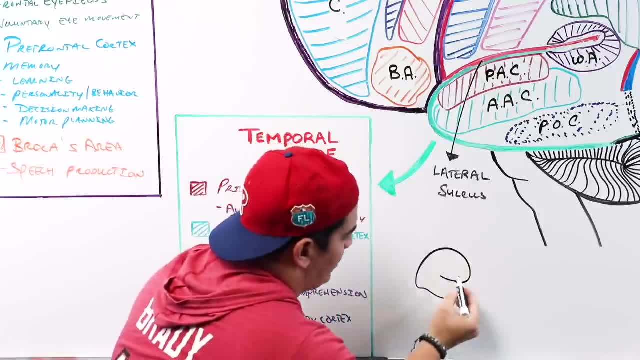 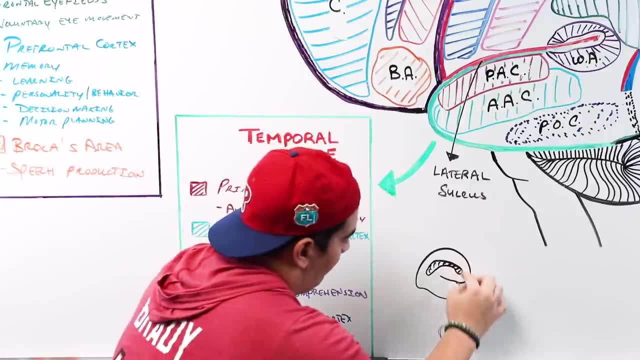 So here's the medial surface And the best way I like to you know, identify that is: you have your corpus callosum here, right? So here would be your corpus callosum And again here would be your frontal lobe. You'd still have a part of that central sulcus coming down here, parietal occipital. sulcus right. But right here is that lateral sulcus And the actual primary olfactory cortex sits just kind of underneath that right And particularly on the medial aspect of the temporal lobe. So that is where the olfactory cortex is located And that's where the temporal lobe is. 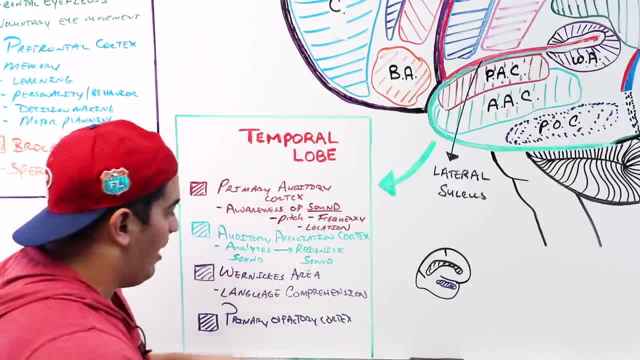 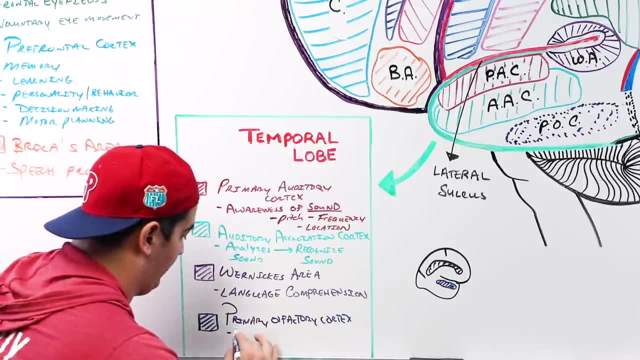 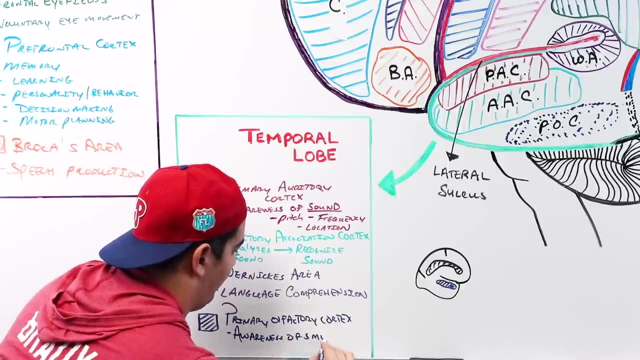 actually located Now, the primary olfactory cortex- and it's an association cortex- is responsible for what? Awareness of smell. And again, that would be the primaries function. So awareness of smell. But again, if you dug in a little bit deeper, the association cortex would be. 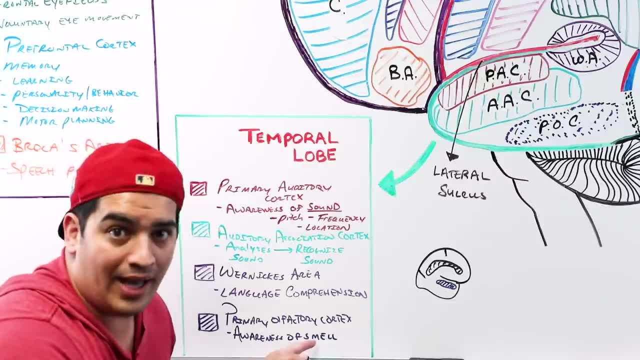 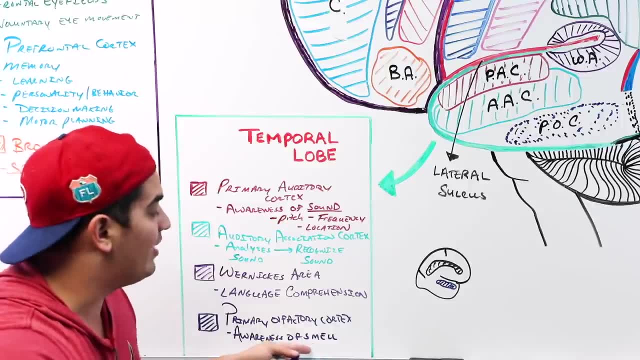 responsible for what? Analyzing the smell and recognizing the smell. So is this a smell of a? you know someone cracking a rat or passing gas or cutting the cheese or farting right? You'd be able to tell that because your association cortex is comparing that smell with past memories of 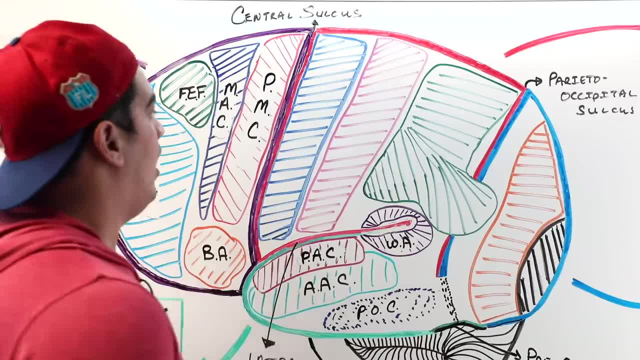 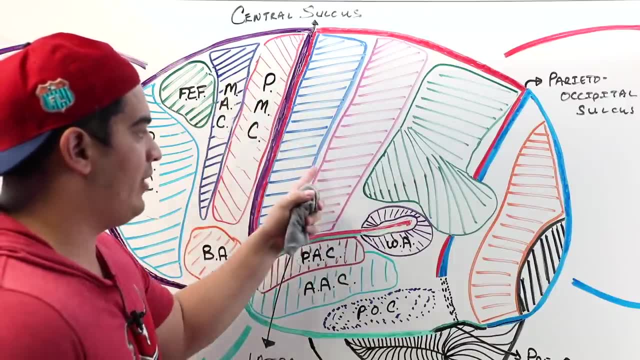 smell. All right, beautiful, That covers the temporal lobe, All right. so now let's talk about the parietal lobe. And again we have that central sulcus, beautifully separating parietal from frontal, as a reminder, and the lateral, separating the parietal from the temporal, and then the parietal 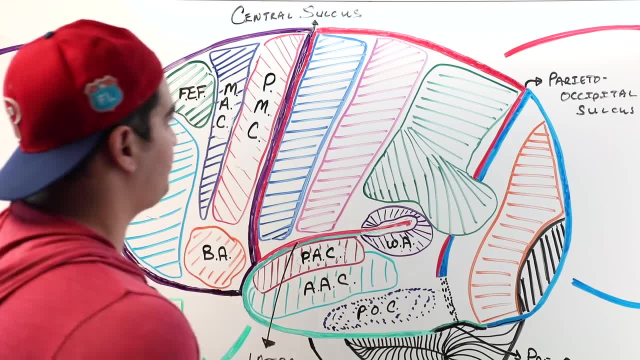 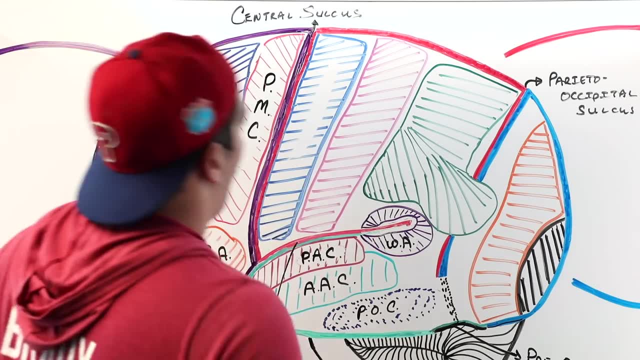 occipital separating the parietal from the occipital lobe- Beautiful Again. just posterior to that central sulcus, and then the parietal occipital separating the parietal from the parietal, you have another gyrus. This is actually called your post-central gyrus. But what I want 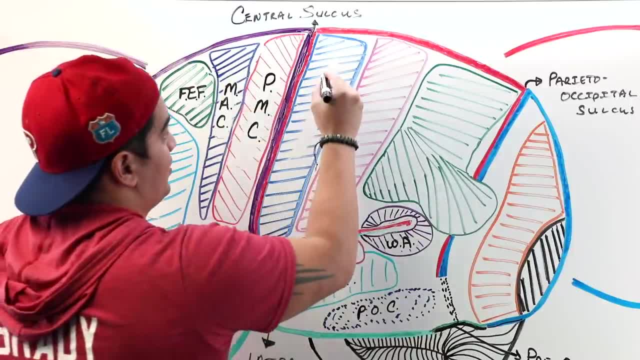 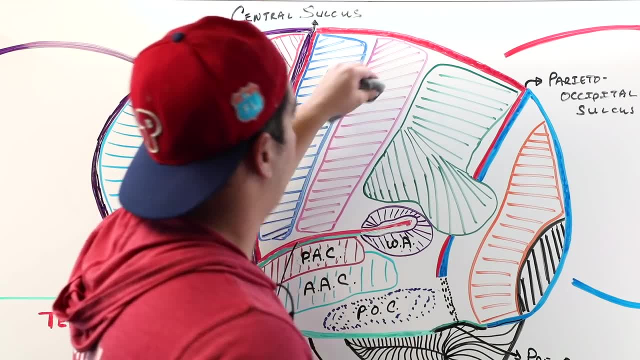 you to remember is that the functional area on that post-central gyrus is called your primary somatosensory cortex. Okay, just posterior to the primary somatosensory cortex, what do you think it's going to be? You guys have already noticed that whenever there's a primary, there has to be 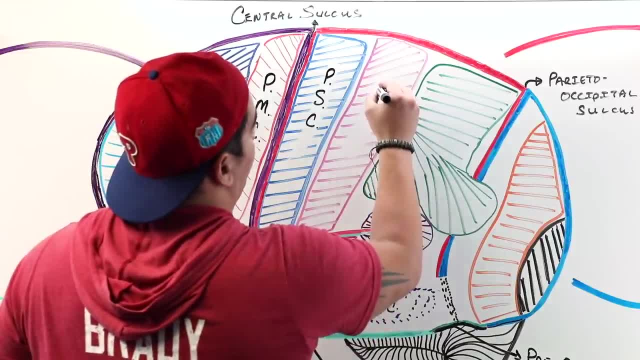 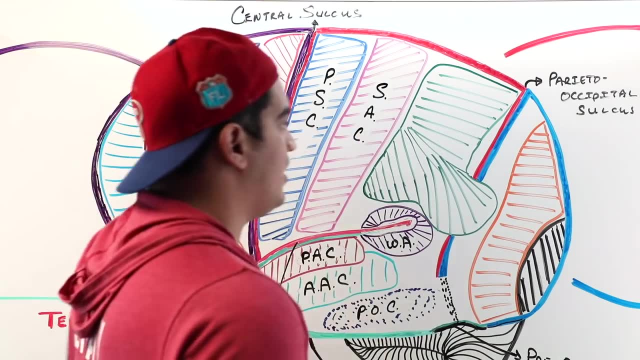 an association cortex, So this is actually going to be called the somatosensory association cortex- Beautiful. Then just posterior to the primary somatosensory cortex, you have another gyrus, So just posterior to that is a very weird area that I felt like we're going to talk about, and 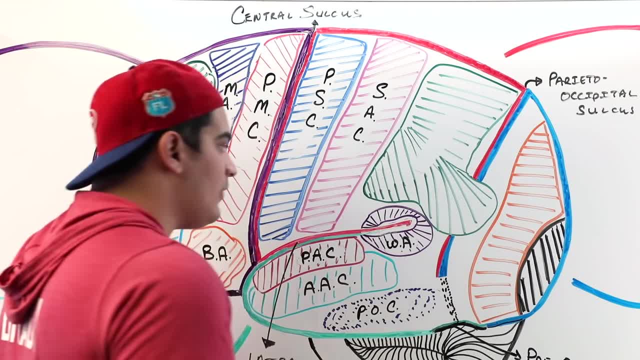 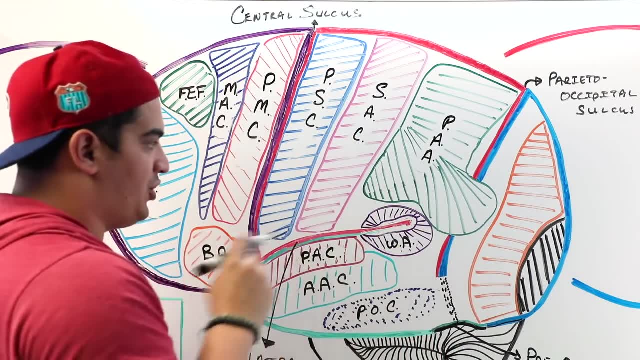 really more particularly discuss it within the parietal lobe. This is actually called the posterior association area. It's a multimodal association area and I'll explain what that means in a little bit. But these are the areas that we're going to focus on. okay, within the 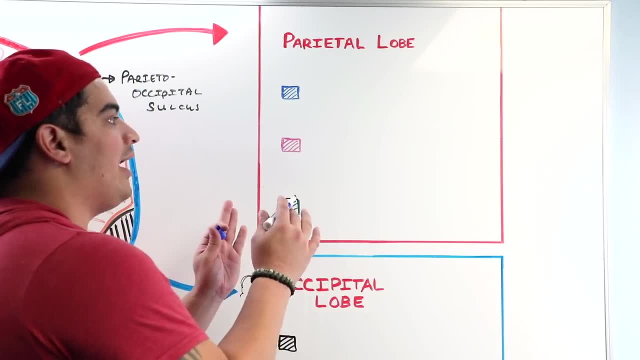 parietal lobe. Now let's talk about their function. All right, so when we talked about the parietal lobe, again just posterior to that central sulcus, we had what's that first kind of area We call it. 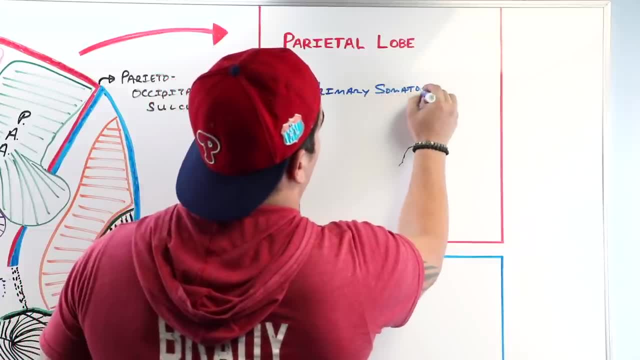 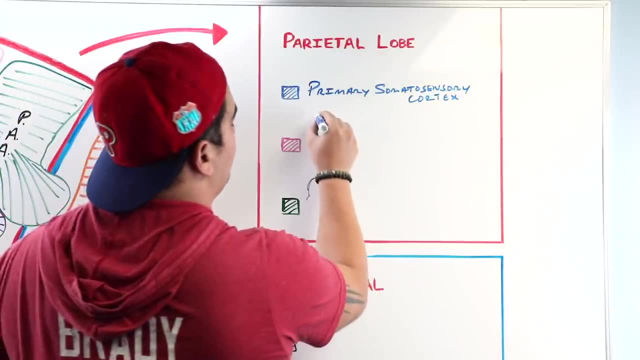 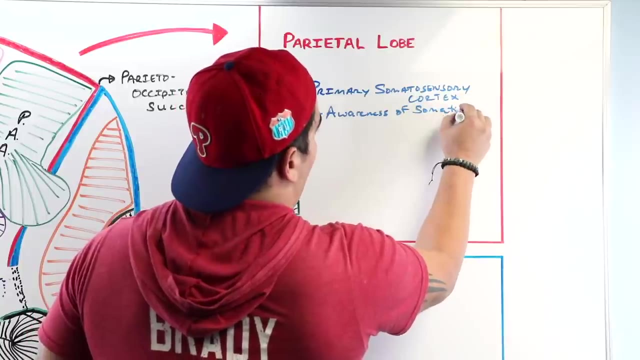 the somatosensory cortex right And again. I just want you guys to kind of look at like a one liner of what it does. The primary somatosensory cortex is involved in awareness of somatic sensations. Now to expand on that, what does that mean? That means fine touch, discriminative touch. 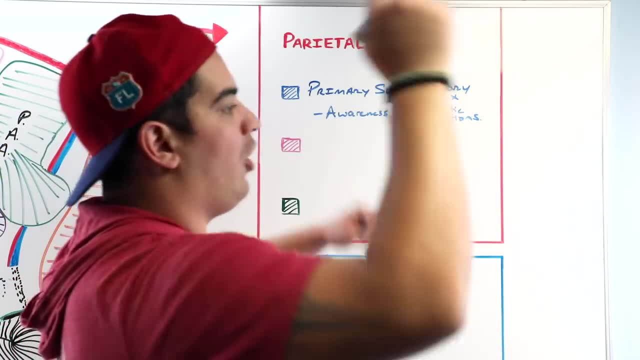 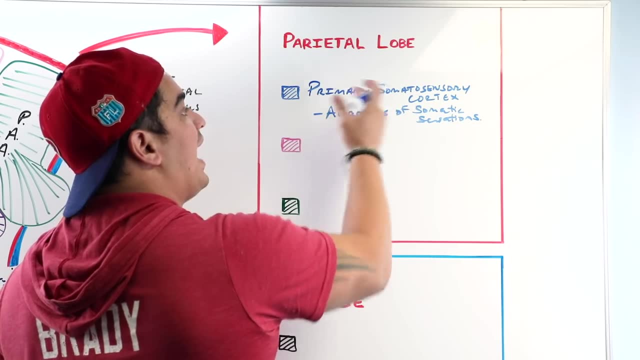 It means proprioceptive sensations, which is where your body, your arm, your body parts are in a three-dimensional space, and even vibration, sense and pressure. All of that stuff comes to this area of the cerebral cortex, and so you're aware of those. 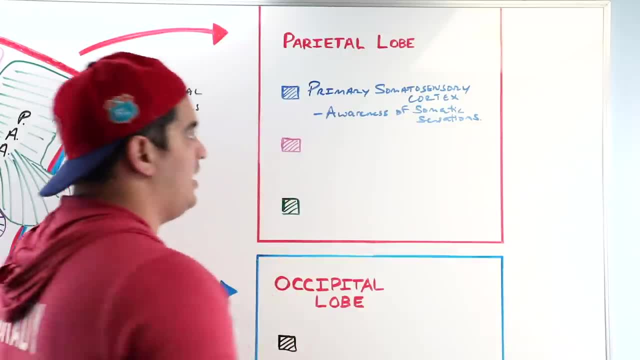 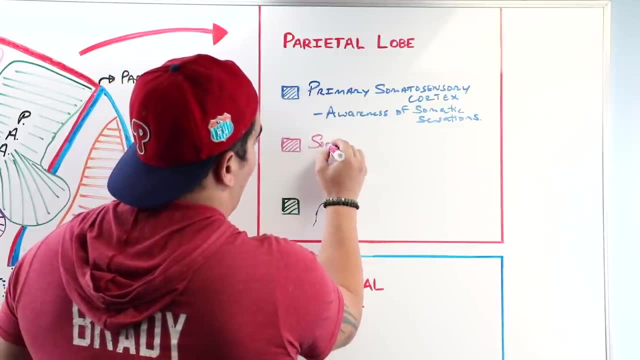 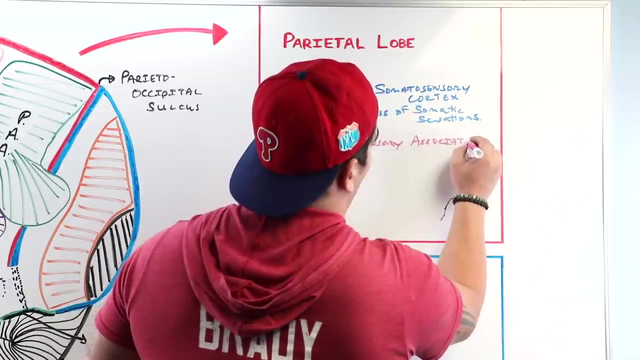 sensations. Now, just posterior to that is an even cooler function. And again, what we say was just posterior to the somatosensory cortex, the primary one, it was the somatosensory association cortex, And I think you guys should at this point start to be seeing a trend here that, anywhere there's, 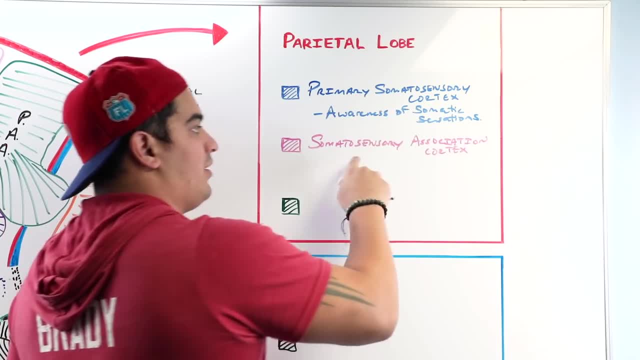 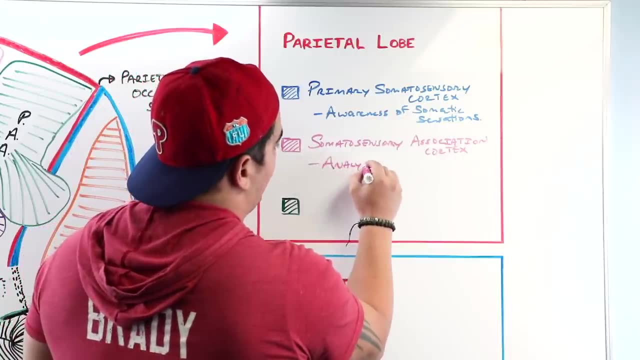 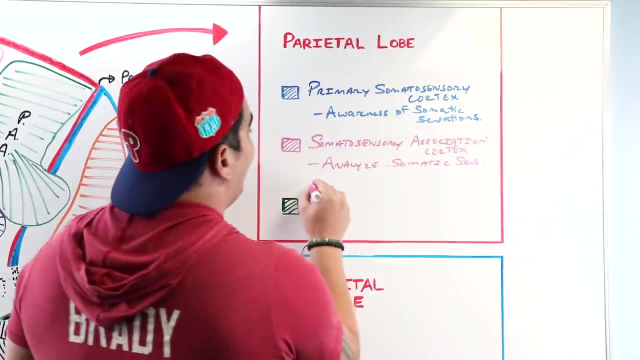 a primary cortex. there's just kind of a highway system that funnels into their association cortex. And this somatosensory association cortex will then do what? Well, it'll analyze the somatic sensations. And not only that, but it'll also do what It'll help with the recognition. 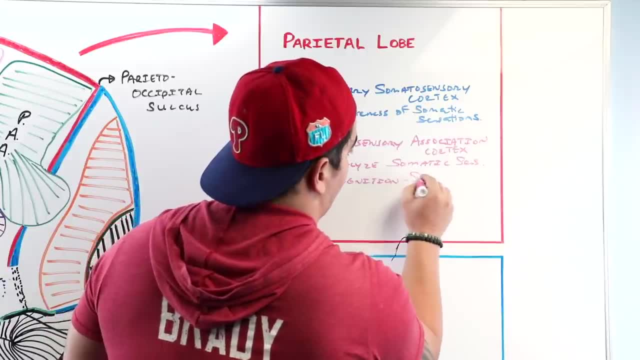 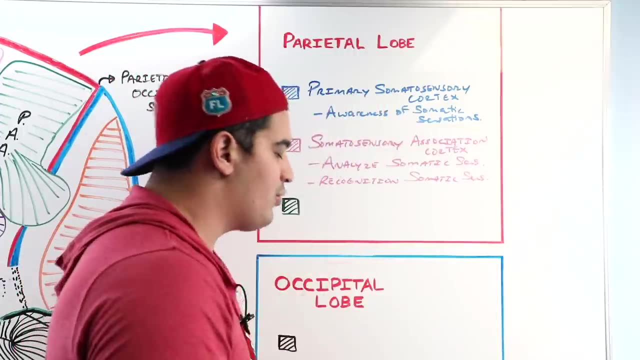 of those somatic sensations. So to give you guys a very simple example here is that if I close my eyes- so I'm not depending upon visual stimulus, right- And someone puts a marker in my hand, I can feel that the marker's in my hand, I can feel that the marker's in my hand, I can feel. 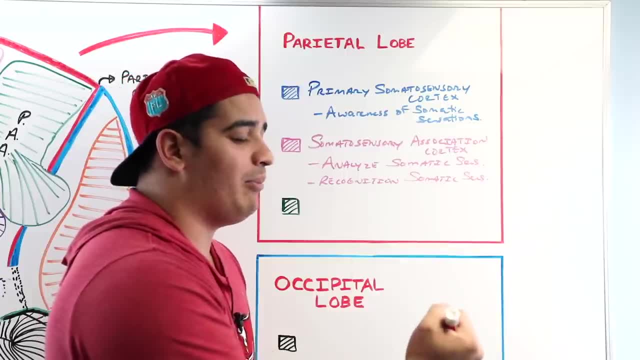 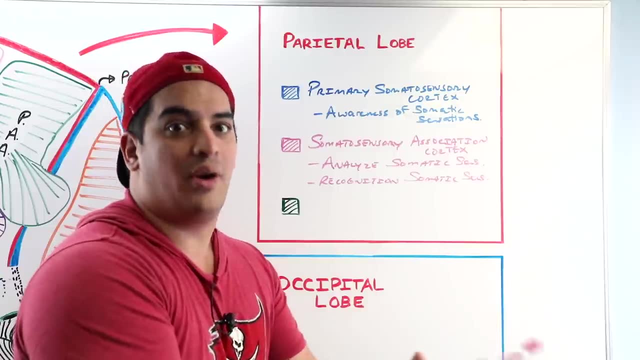 that the marker's in my hand. So that's the sensory pathways. I can also tell that it's in my right hand because of my proprioceptive sensations, And, if I'm pretty good, I can also tell that this is a marker without actually knowing that I'm the one who put it in my hand. So that is what this somatosensory 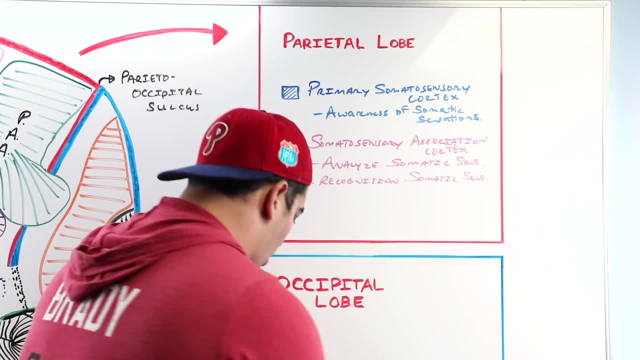 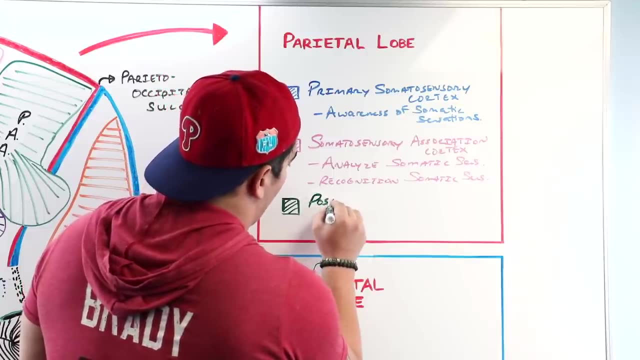 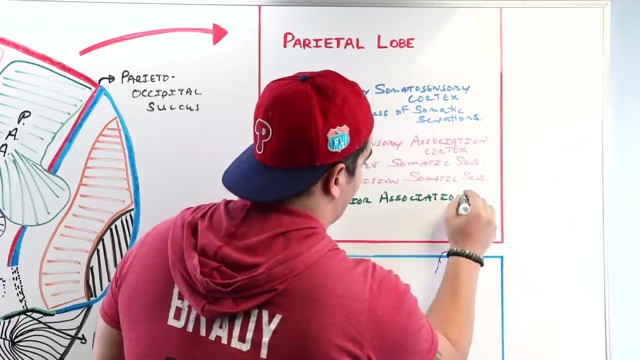 association cortex does is pattern recognition. Okay, The one just posterior to it is the really interesting and weird area. It's called the posterior association area. Now, this area is kind of what we already kind of just explained what it is. I'm going to write it down. It's called: 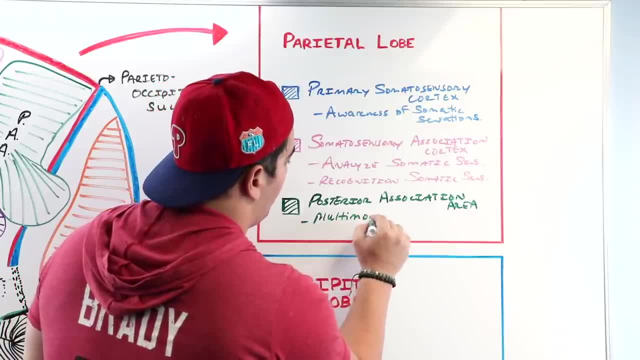 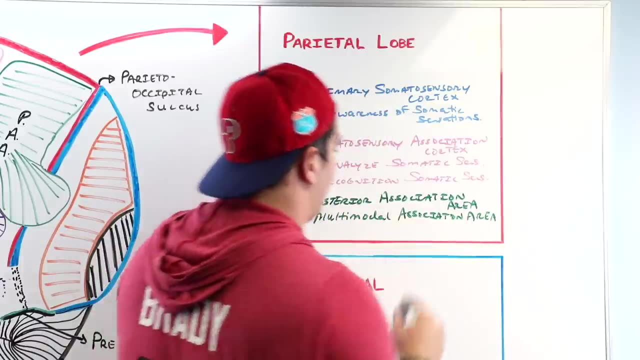 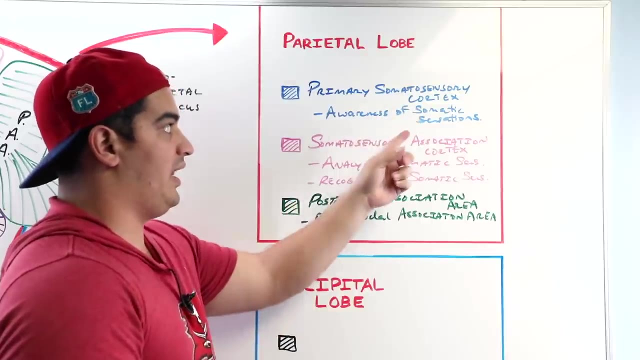 a multimodal association area, And I'm going to very briefly explain what the heck that means. All right, Anytime you guys have noticed a trend here, you have a sensation. Let's take for the example the somatosensory cortex. the somatic sensations go to this area, Then they go to an 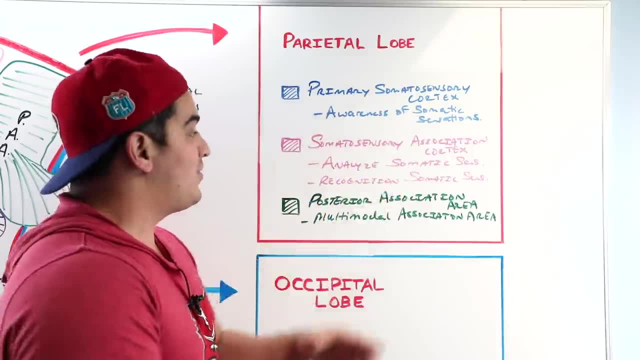 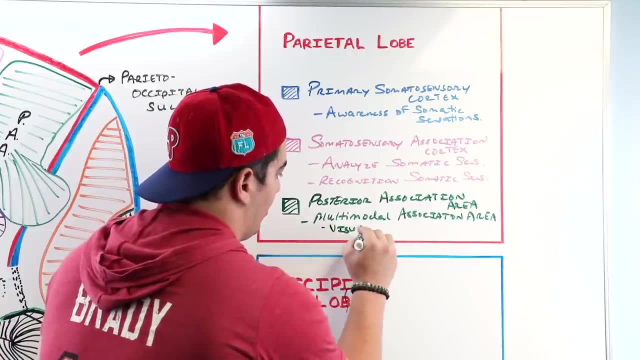 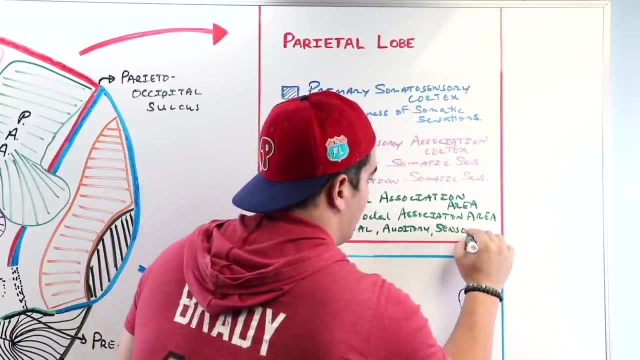 association cortex to be analyzed and recognized. And then they go to an association cortex to be recognized. Well, guess what? What happens is the association cortexes from your visual pathway, your auditory pathway and your sensory pathways all kind of coalesce into one area. So your visual 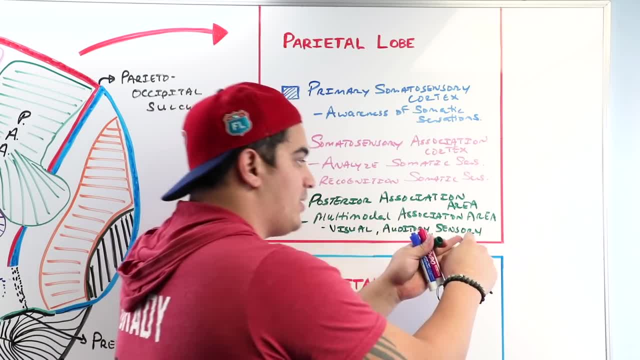 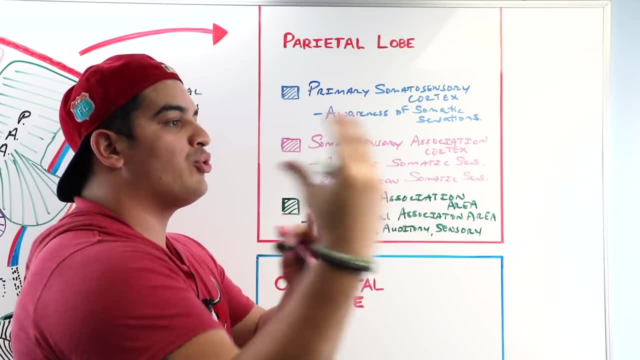 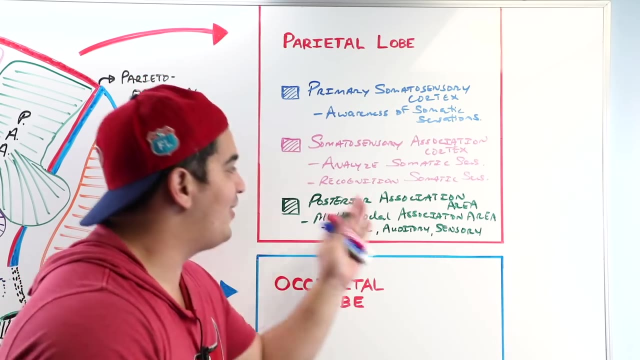 association cortex, auditory association cortex and somatosensory association cortex then funnel their influence to the posterior association area. Now I can determine a sense of spatial coordination of visual stimuli, auditory stimuli and sensory stimuli. That is the function of this beautiful area And it can communicate with a bunch of other areas. 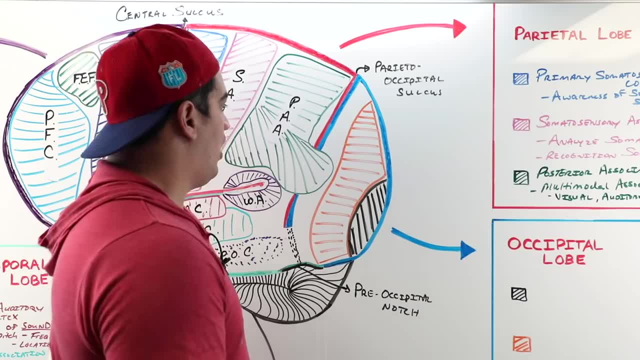 in the brain. All right, Beautiful, That covers a parietal lobe, All right. So now we got our last lobe here, that we got to talk about the occipital lobe, right And again, what did we say was the? 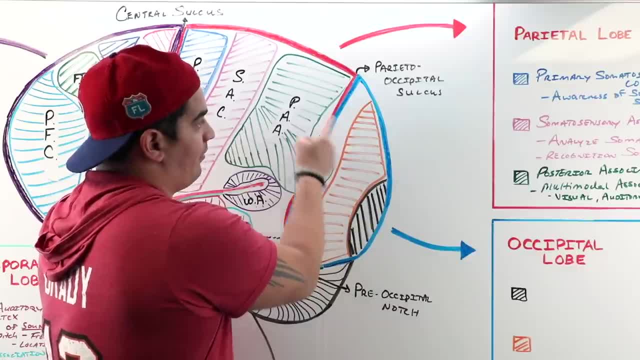 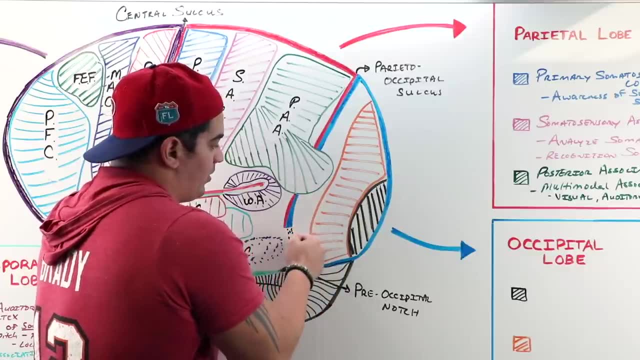 demarcation points. We had the parietal occipital sulcus, which separates it from the parietal lobe, and that imaginary line coming from the preoccipital notch that comes and meets the occipital sulcus, separates the occipital from the temporal. All right, We got two cortex in this. 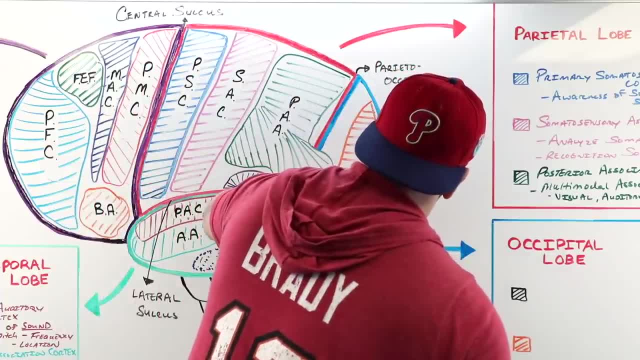 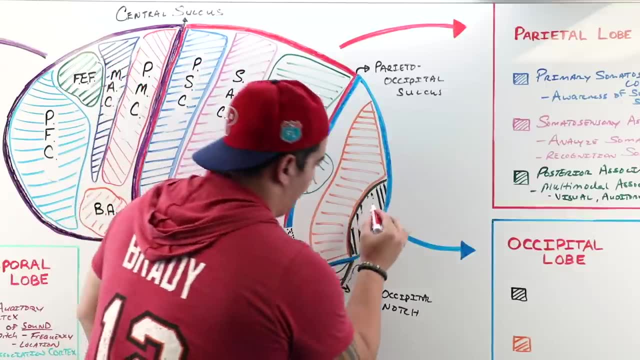 area, two areas, particularly One. we're going to start with this one most posteriorly. Okay, This one right here is actually referred to as- let's do it in red, so we can really differentiate it. This one is called your primary visual cortex. Now, if you go just 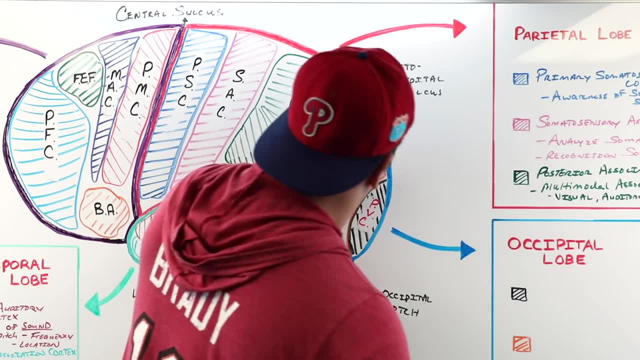 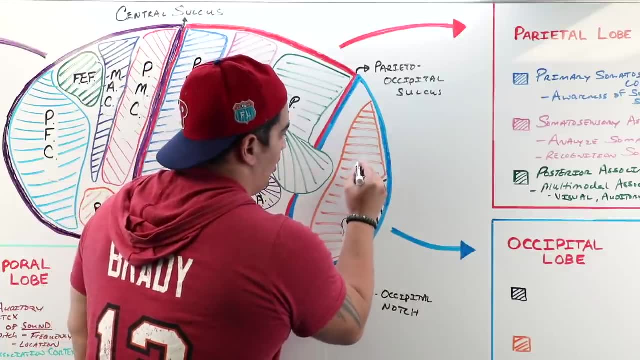 anterior to the primary visual cortex, you have another area And this area again. you guys should already get the point of this: Wherever there's a primary, there is an association. So this is called your visual association cortex. All right, That covers the areas. Now let's go. 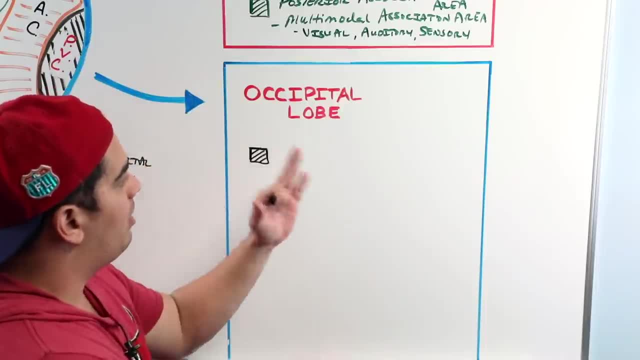 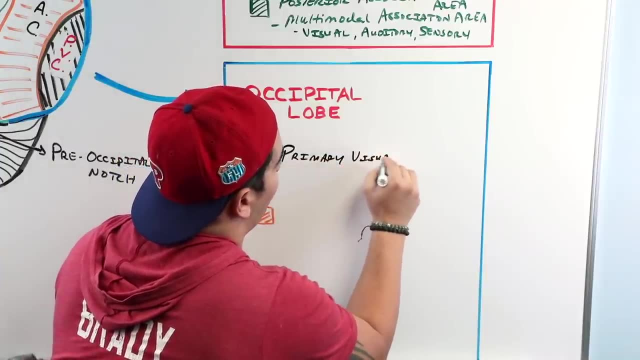 ahead and talk about their function. All right, Beautiful, So occipital lobe. Now let's talk about the functions of those areas. What were the first area that we talked about? The primary visual cortex. right And the primary visual cortex. what did we say it was responsible for? 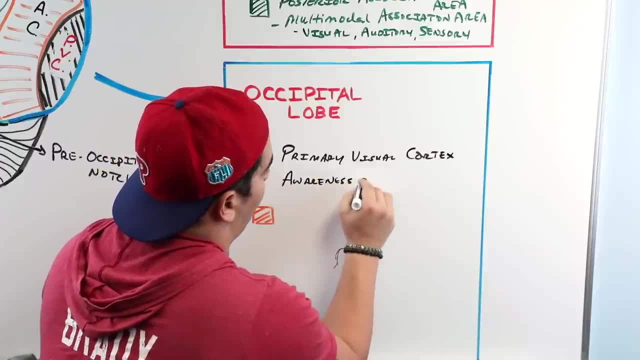 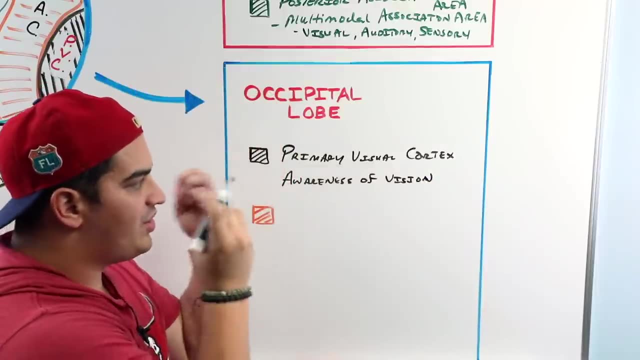 Awareness, So conscious awareness of vision, right. So a visual stimulus, if you will. Now, when the visual stimuli comes from your eyeballs right And then goes to your occipital lobe and your primary visual cortex, then it has. 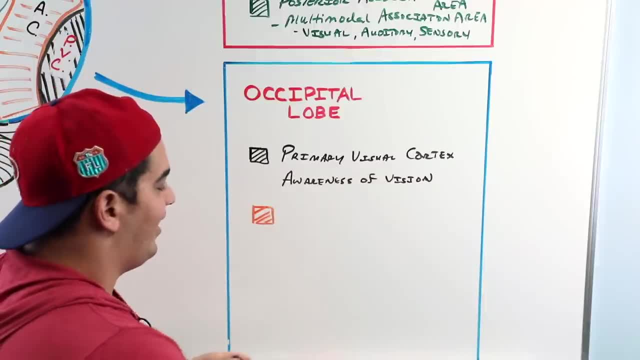 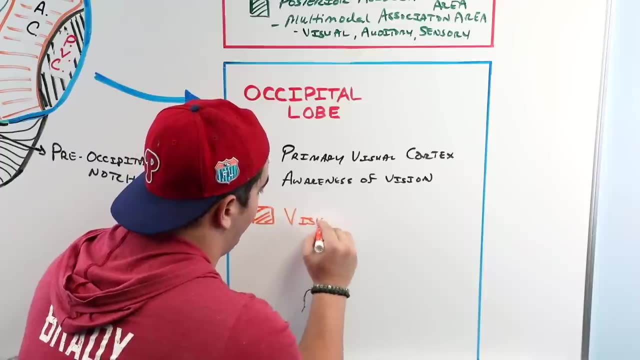 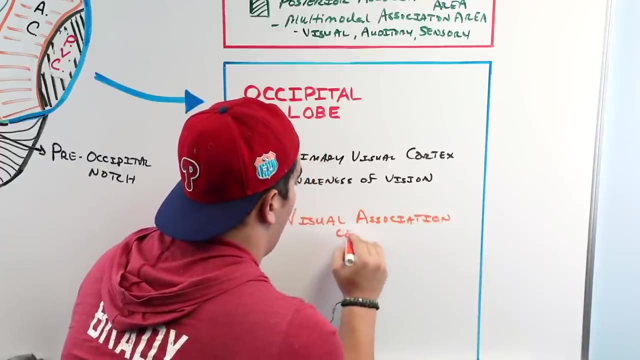 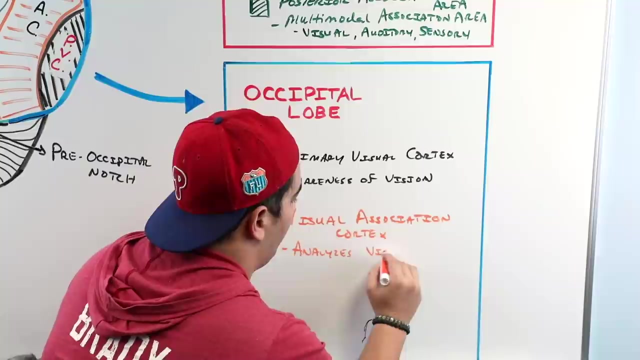 to go to what other structure? What's the highway system for the other structure that it moves into? It then goes into the association cortex. So the next one, which was just anterior to it, is called the visual association cortex. And again, what does this do? It analyzes the visual stimulus, All right. So how does it? 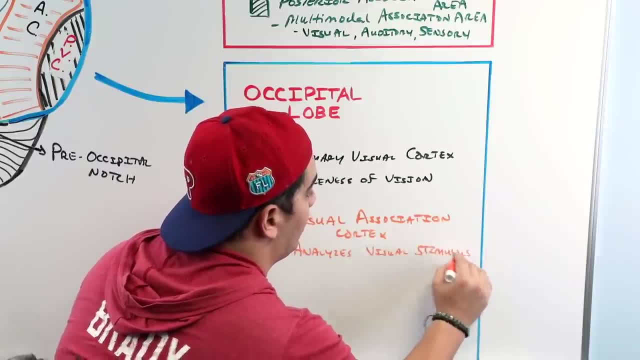 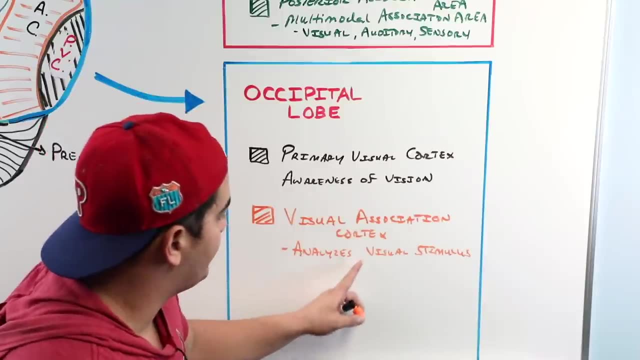 how does it do that? Well, it takes the visual stimulus and it looks at the color. Maybe again, this is orange. I'm telling that because of my visual association cortex. It also tells me the angles right Of how I wrote V, how I kind of wrote I. It tells me if something's moving. 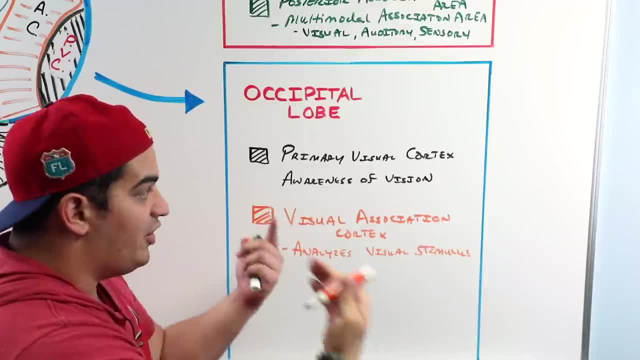 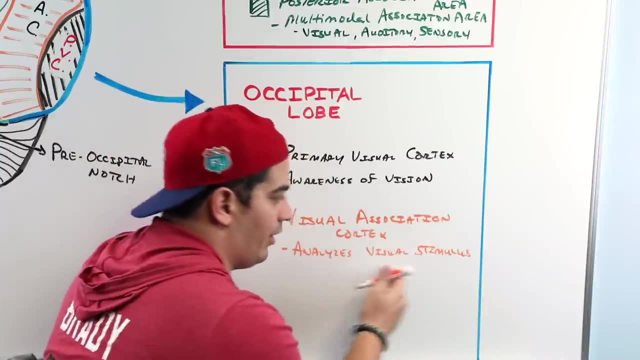 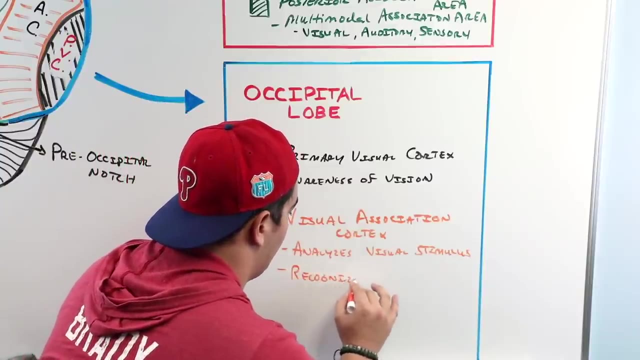 right, Or if it's staying still, All of that stuff, that visual stimulus of all these things is going to go to my primary visual, then to your visual association cortex, where it analyzes the color, the movement, the angles. So it helps us to recognize our visual stimulus right Now. 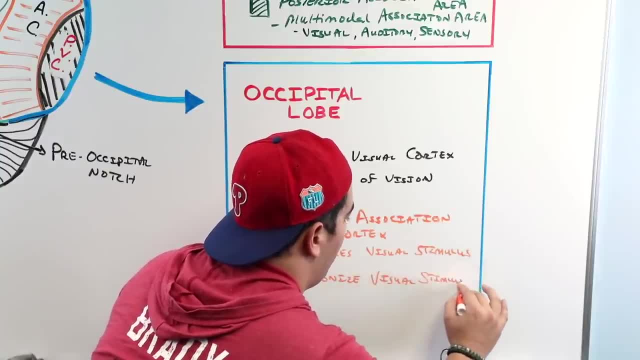 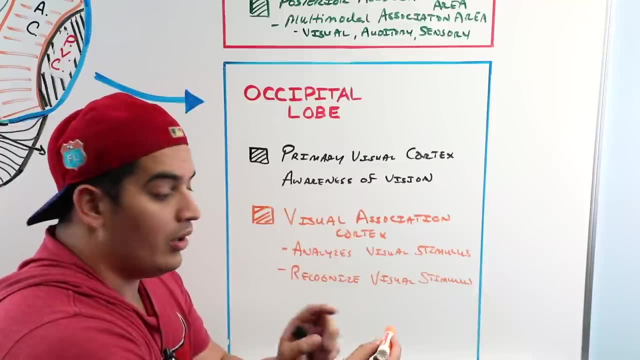 that's really important if you think about the overall concept of that. So, if you think about it, I have a marker here, right? How do I, how am I able to tell that that's a marker? Well, I'm able to tell because I see kind of the shape of it, I see kind of the angles involved in it, I see 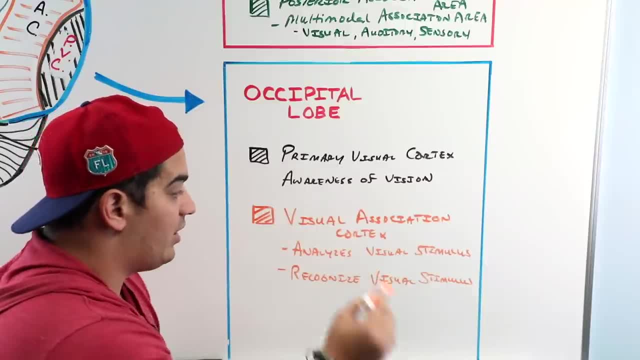 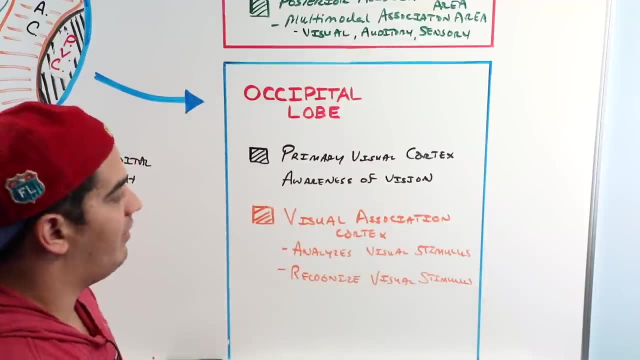 the color that it's an orange marker. I can tell that basically what I can do with it, because the visual association cortex is responsible for that. So that's the beauty of this cortex. All right, that covers our occipital lobe, All right. So I said I wasn't going to cover the insula in this. 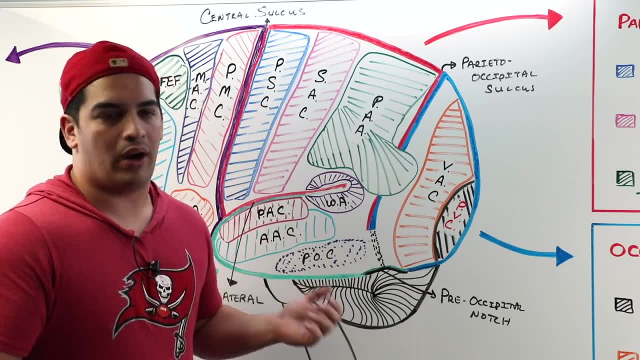 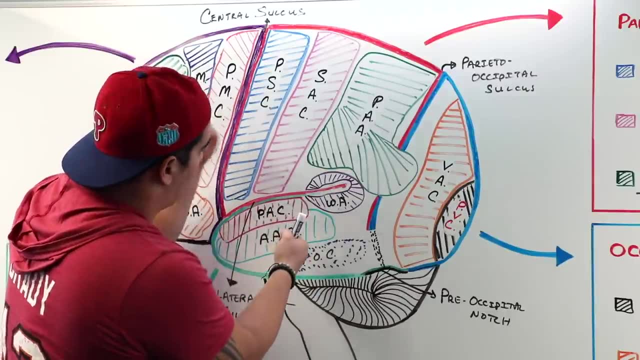 video, but I feel bad. I want to make sure that what you guys know kind of the basic idea of where it is. So imagine I had two hooks. right, I'm going to take a hook and I'm going to stick it into the lateral sulcus. I'm going to yank down. I'm going to take another hook, I'm going. 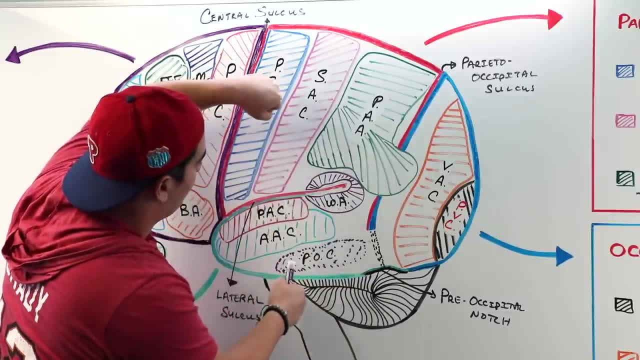 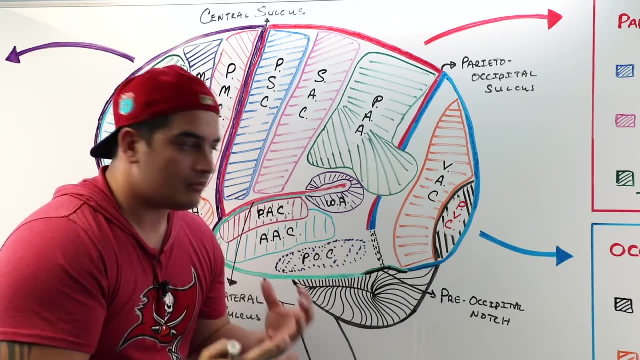 to stick it under the lateral sulcus and I'm going to pull up. If I pull down and pull up, there's going to be a little lobe of brain tissue sitting right here and that's called the insula. Now, what I want you guys to know about the insula is just the. 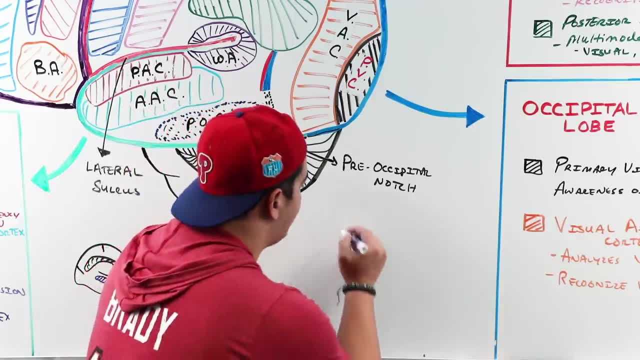 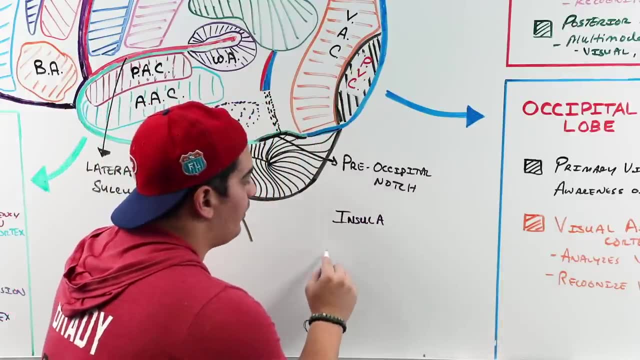 basic functions of the insula. All right, So again, the insula is that structure that we talked about. if we were to kind of pull on that lateral sulcus, right? I want you to know just the three basic functions of the insula. One is that it is responsible for receiving taste. 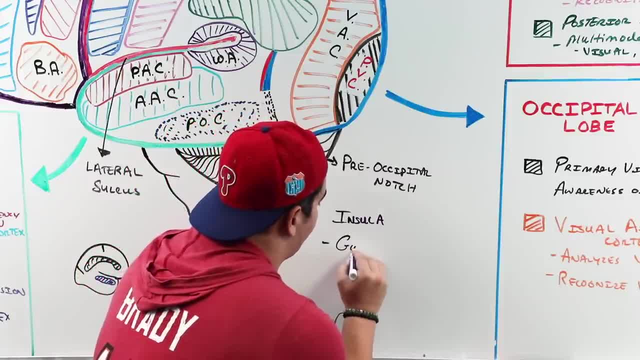 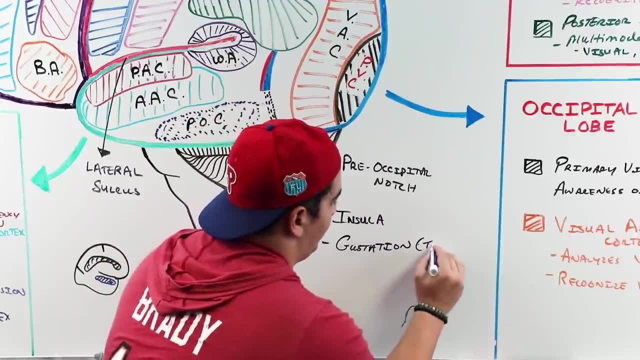 sensations. So it's involved in gestation. So this might be where your gestation cortex is actually located. So gestation is also known as taste. Let's just write that down. It's known as taste, So this is where taste is taken to, So we're aware of taste. and then the association gestation. 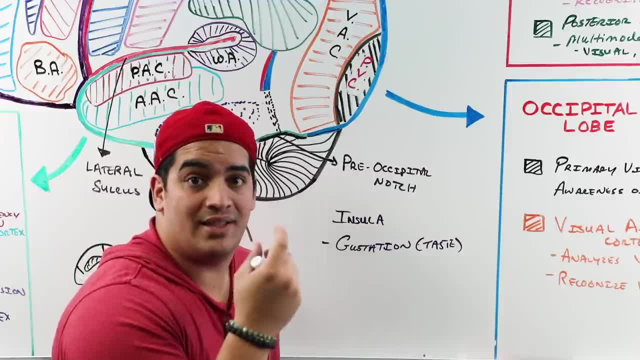 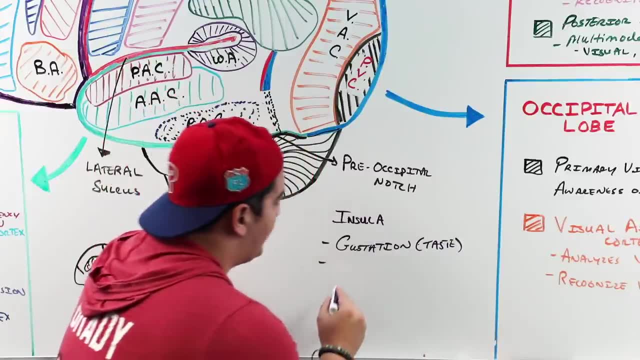 cortex would be involved in what, Telling us what kind of taste it is, If it's sweet, if it's sour, if it's bitter, if it's salty or if it's umami. And the other function of the insula is it's. 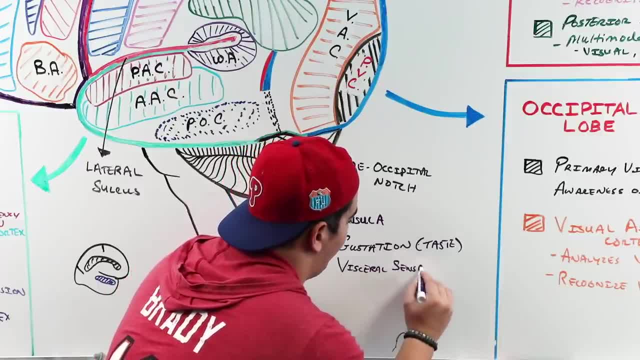 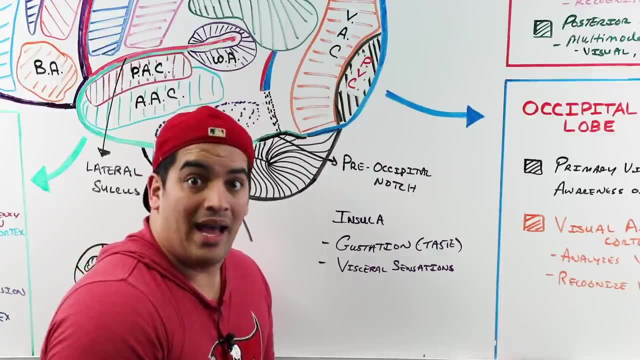 being aware of our visceral sensations, So sensations coming from the GI tract, the heart, the lungs, things of that nature. If you guys have ever had gastroenteritis, the pain from that- right, So just a GI bug, the pain from that GI tract will go to your insula and make you aware.